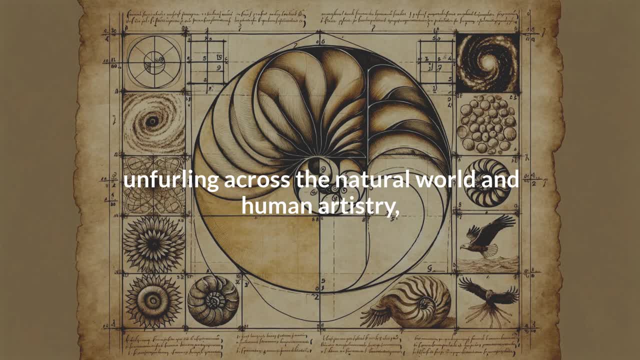 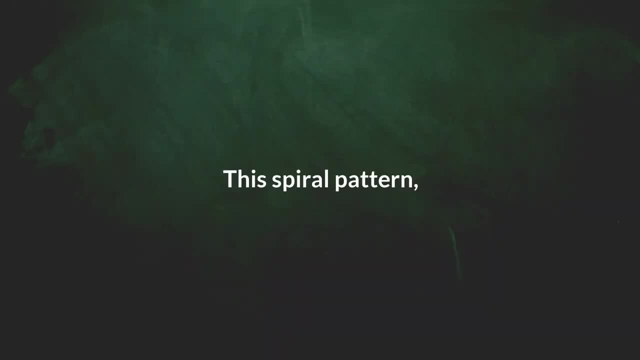 unfurling across the natural world and human artistry, offering a mesmerizing glimpse into the harmony of the universe. This spiral pattern, born from the Fibonacci sequence, where each number is the sum of the two preceding ones, reveals an astonishing mathematical order underlying life itself. 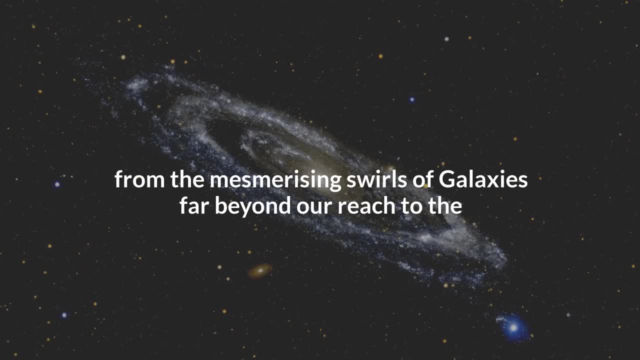 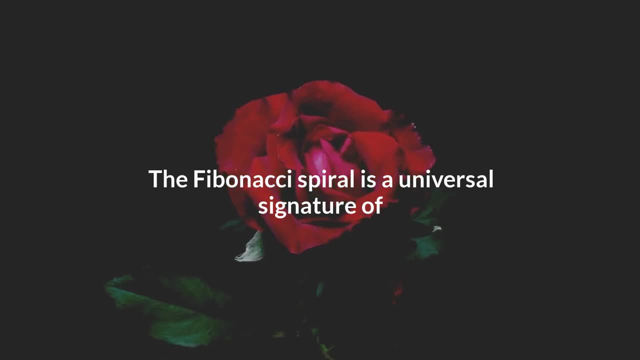 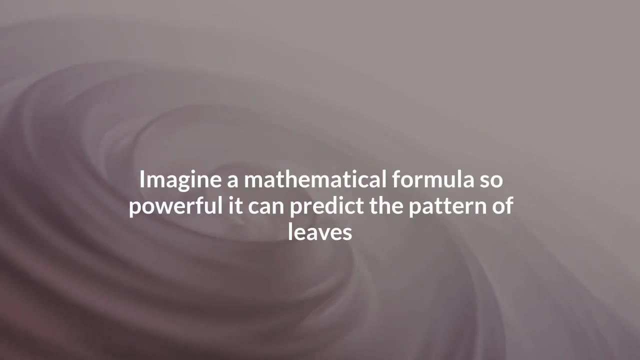 From the mesmerizing swirls of galaxies far beyond our reach to the delicate unfurling of a rose's petals, the Fibonacci spiral is a universal signature of beauty and balance. But why is it so utterly fascinating? Imagine a mathematical formula so powerful it can predict the pattern of leaves around a stem. 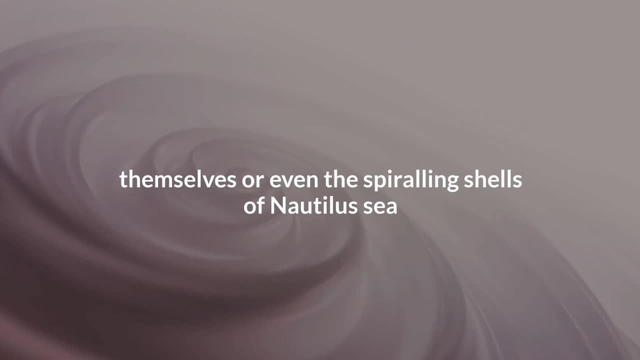 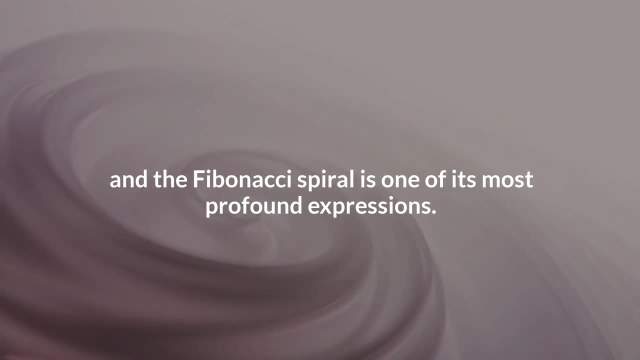 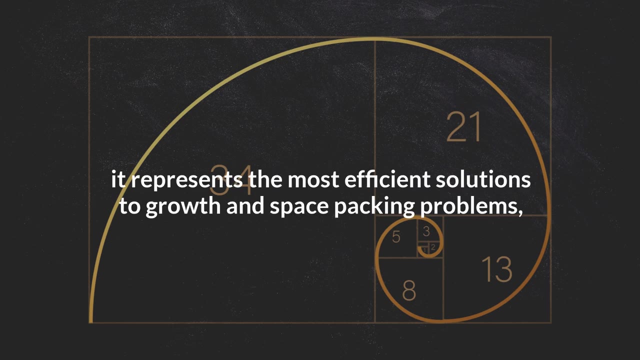 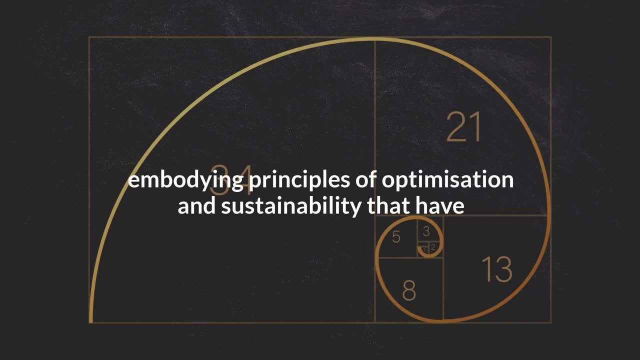 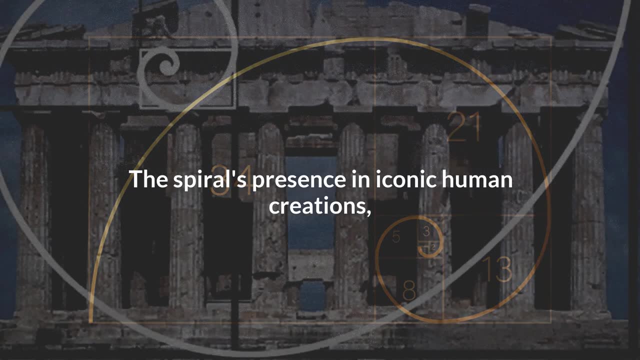 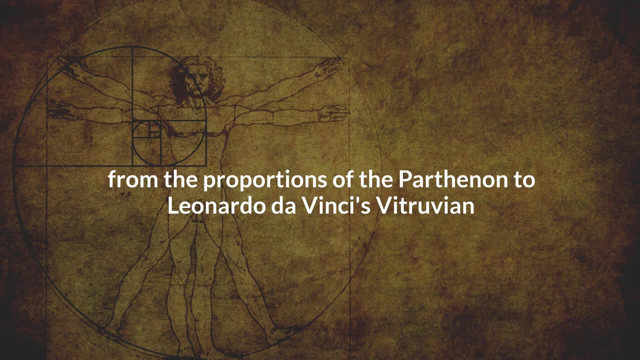 embodying principles of optimization and sustainability that have inspired artists, architects and designers for centuries. The spiral's presence in iconic human creations, from the proportions of the Parthenon to Leonardo da Vinci, to the evolution of the world, to Leonardo da Vinci's Vitruvian Man. 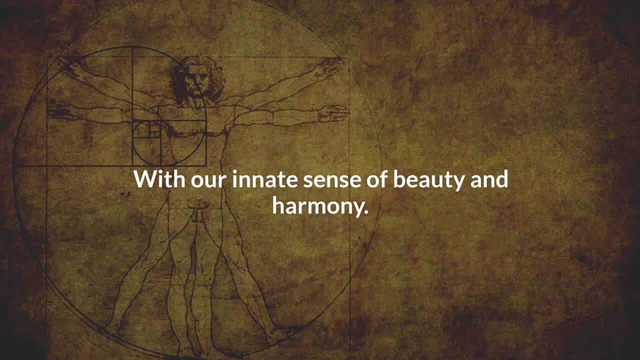 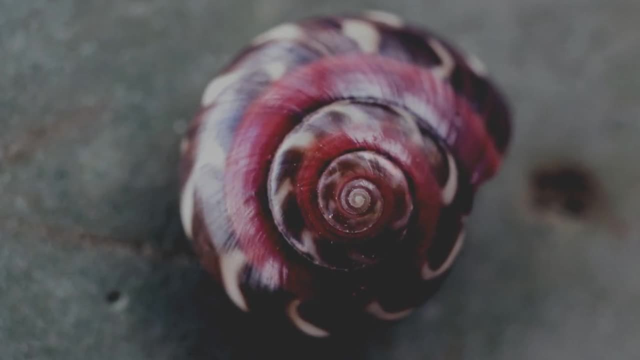 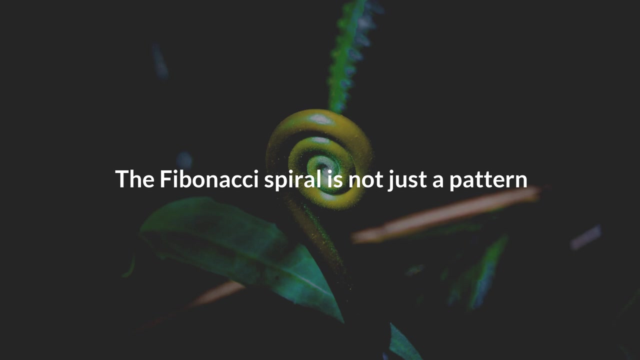 underscores its deep resonance with our innate sense of beauty and harmony. It bridges the gap between the tangible and the mystical, inviting us to explore the deeper connections between all forms of existence. The Fibonacci spiral is not just a pattern. It's a testament to the interconnectedness. 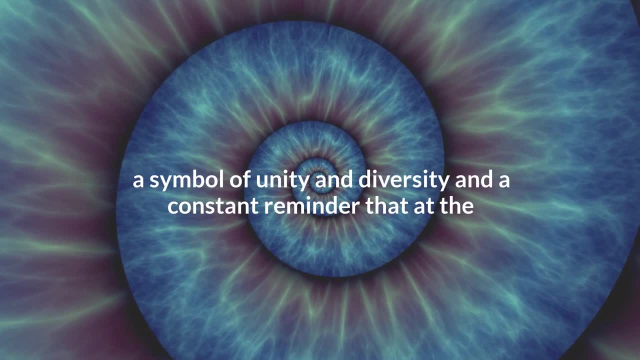 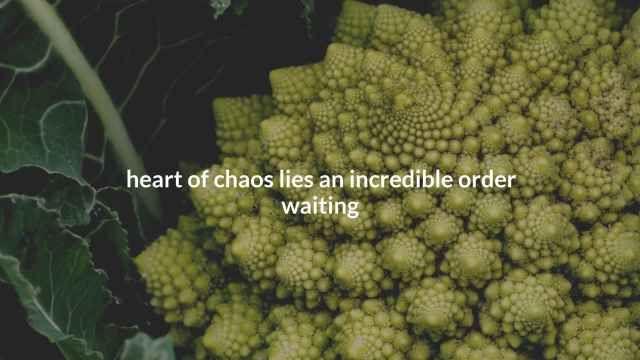 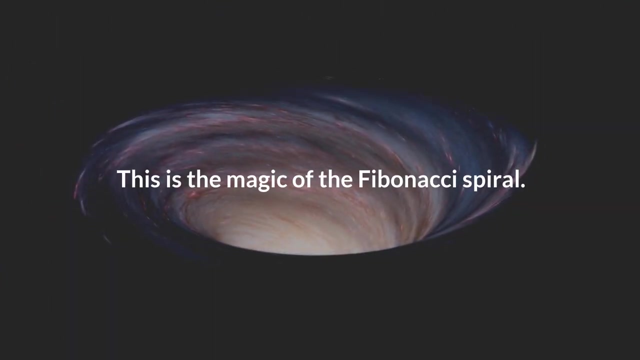 of everything in the cosmos. It's a symbol of the universe, A symbol of unity and diversity and a constant reminder that at the heart of chaos lies an incredible order waiting to be discovered. This is the magic of the Fibonacci spiral in sacred geometry. 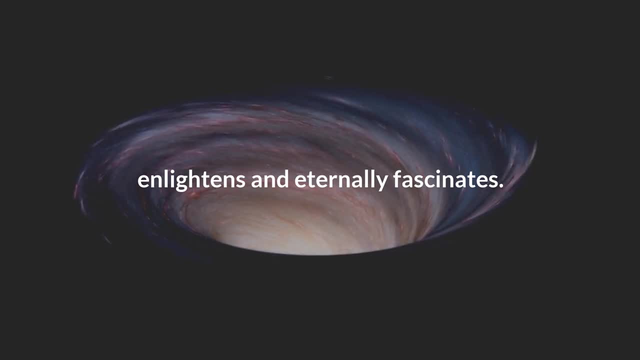 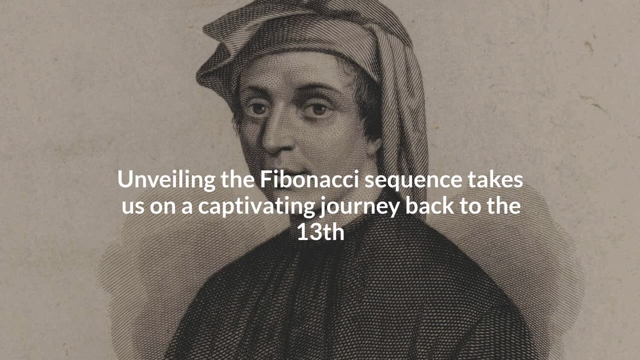 It enchants, enlightens and eternally fascinates. Unveiling the Fibonacci sequence takes us on a captivating journey back to the 13th century with Leonardo Fibonacci, an Italian mathematician whose legacy transcends the realm of mere numbers and ventures. 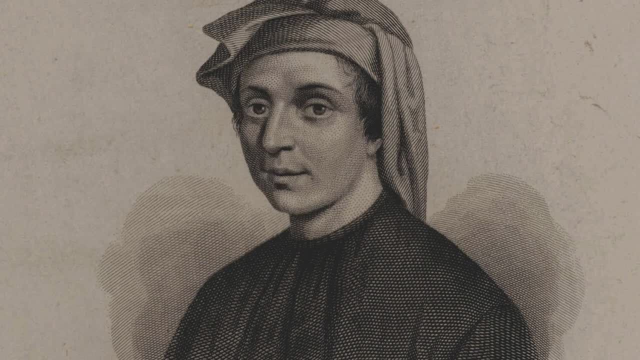 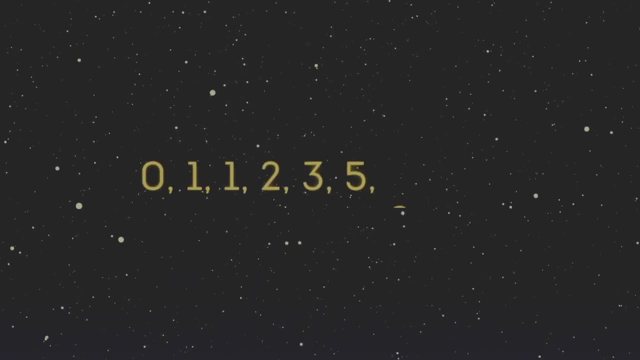 into the profound mysteries of life itself. This sequence seemingly innocuous, with its simple progression from 0, 1,, 1,, 2,, 3,, 5,, 8,, 13, and, beyond each number, a sum of the two preceding ones. 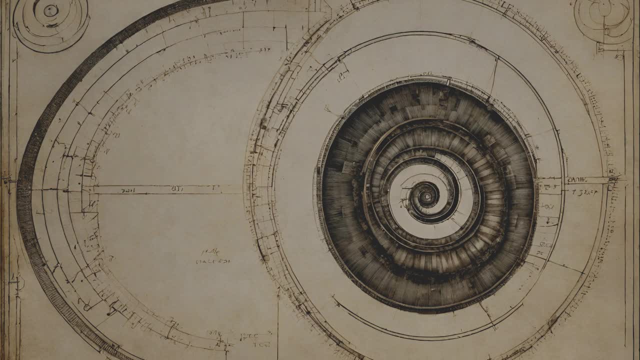 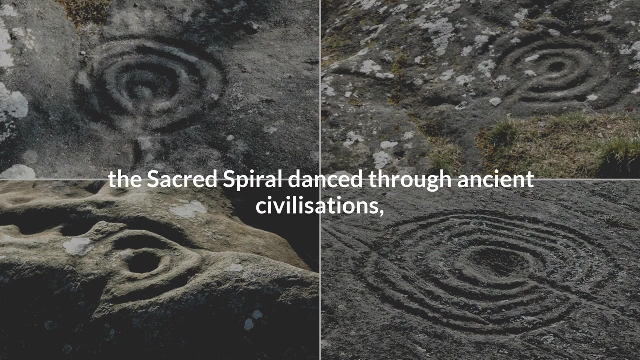 is far more than a mathematical equation. It's a symbol of the universe. It is, in essence, a fundamental pattern underlying the very fabric of existence. However, long before Fibonacci unveiled the sequence that bears his name, the sacred spiral danced through ancient civilizations immortalized in stone. 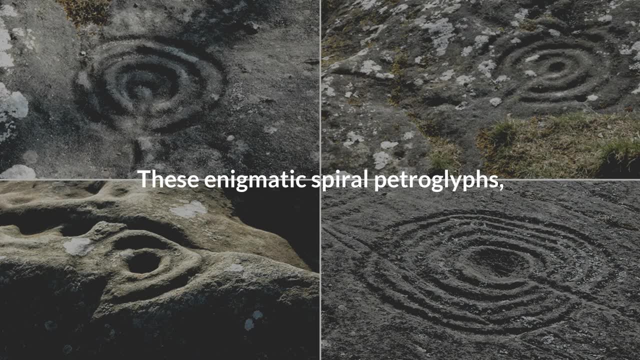 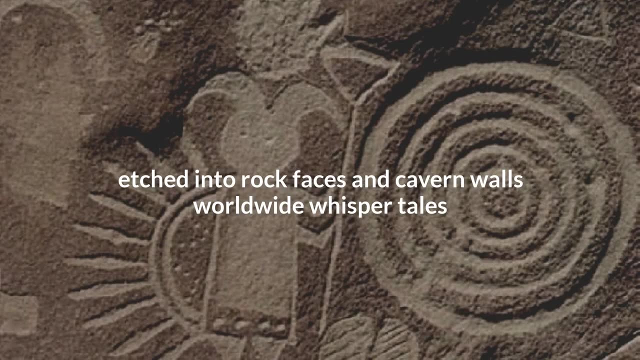 by the hands of our ancestors. These enigmatic spiral petroglyphs etched into rock faces and cavern walls worldwide whisper tales of humanity's age-old fascination with this cosmic pattern, These primordial symbols found from the windswept deserts. 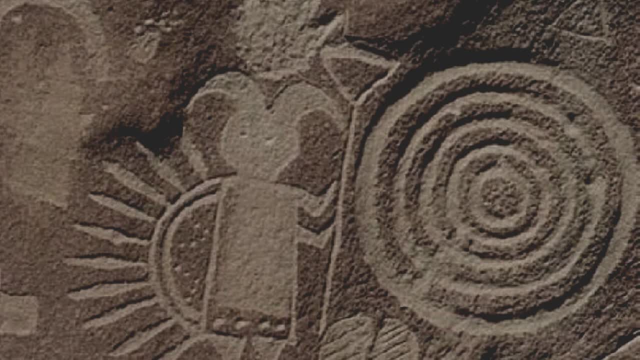 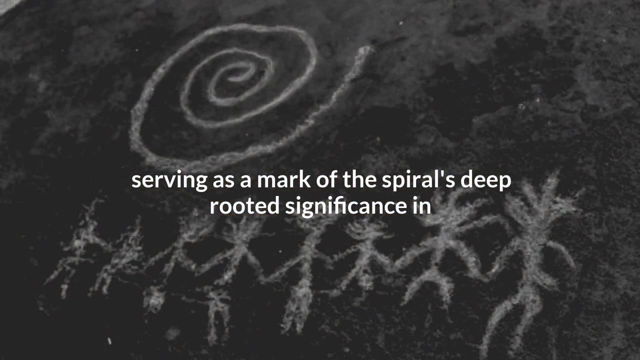 of North America to the mystical shores of Ireland, predate Fibonacci by millennia. serving as a mark of the spiral's deep-rooted significance in human consciousness, They are not mere decorations but profound expressions of the universe's inherent order: a prehistorical 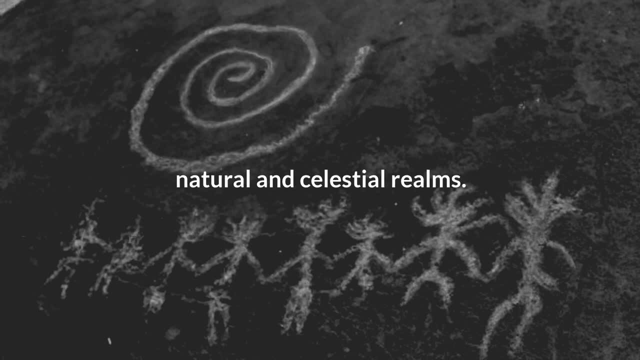 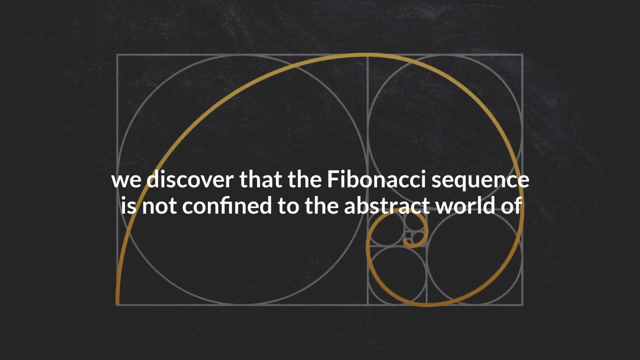 symbolic acknowledgement of the spiral's role in the natural and celestial realms. As we delve deeper into this narrative, we discover that the Fibonacci sequence is not confined to the abstract world of mathematics. Rather, it manifests itself in the most unexpected and diverse aspects of the natural world. 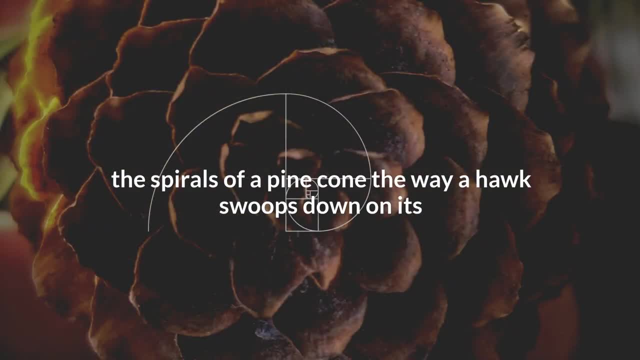 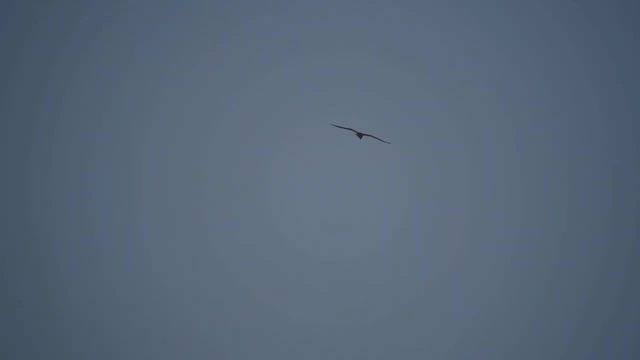 The arrangement of seeds in a sunflower, the spirals of a pine cone, the way a hawk swoops down on its prey- All are guided by this sequence. It's as if nature itself has been coded with this numerical sequence, an underlying blueprint for life's most intricate designs. 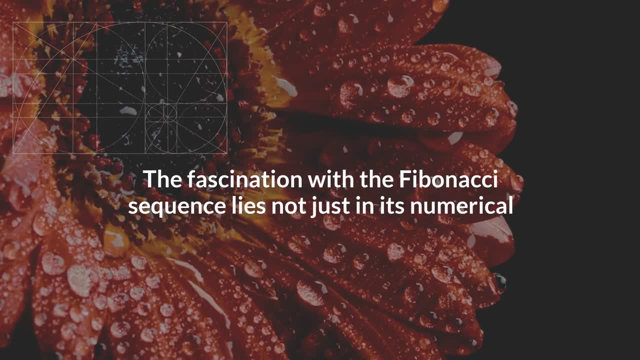 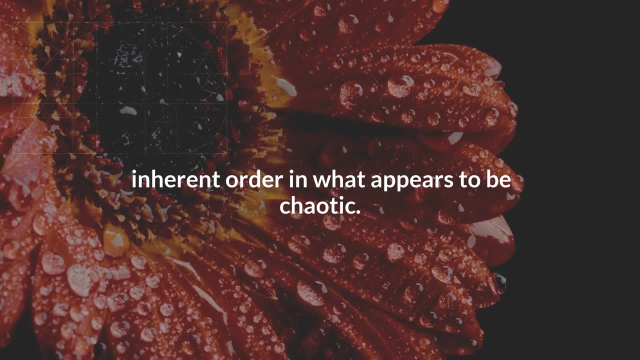 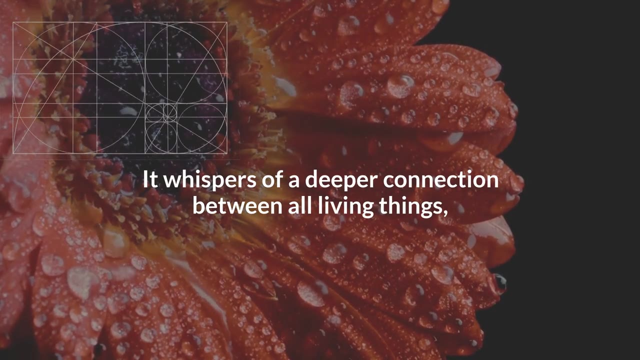 The fascination with the Fibonacci sequence lies not just in its numerical beauty, but in its universality and its ability to reveal the inherent order in what appears to be chaotic. It whispers of a deeper connection between all living things, a sort of mathematical kinship. 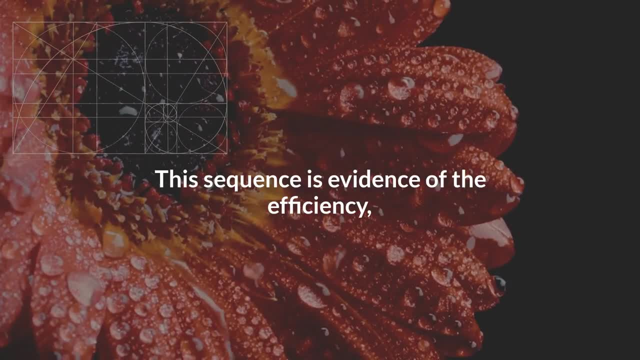 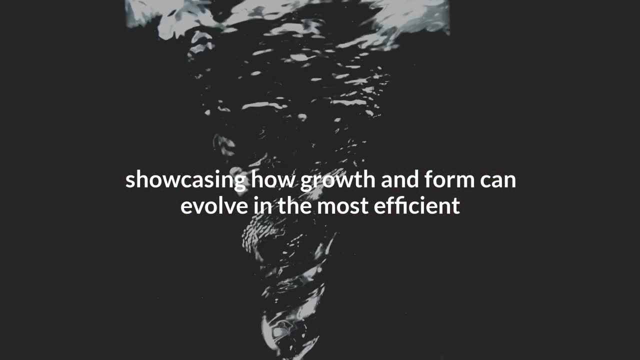 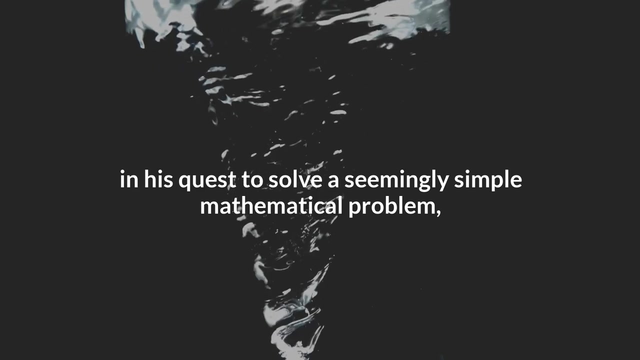 that binds the cosmos. This sequence is evidence of the efficiency, adaptability and elegance of natural selection, showcasing how growth and form can evolve in the most efficient patterns. Leonardo Fibonacci, in his quest to solve a seemingly simple mathematical problem, unveiled a principle. 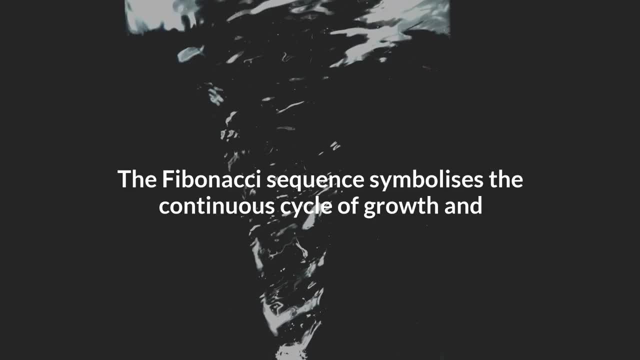 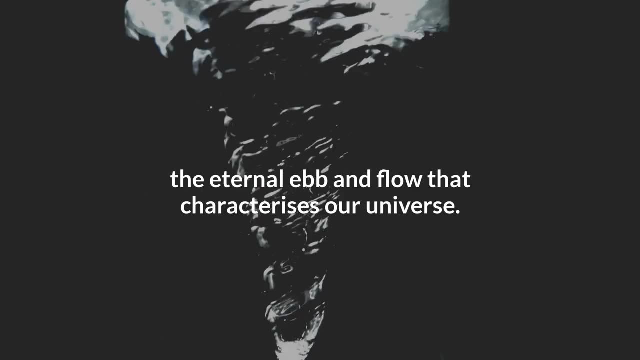 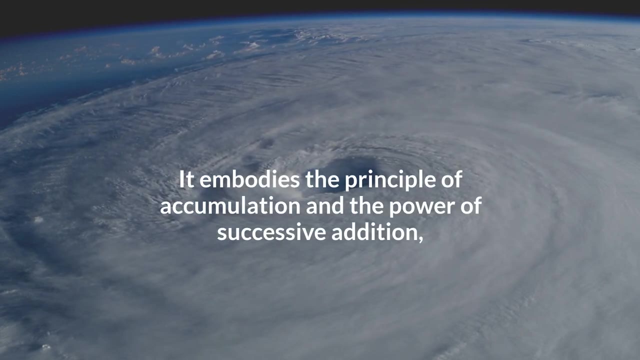 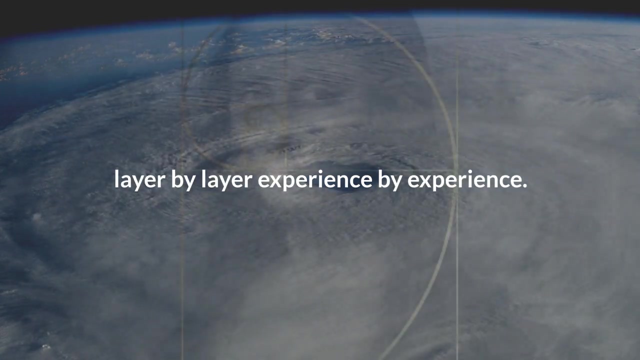 that stretches far beyond numbers. The Fibonacci sequence symbolizes the continuous cycle of growth and decay, the eternal ebb and flow that characterizes our universe. It embodies the principle of accumulation and the power of successive addition, mirroring the way life builds upon itself, layer by layer, experience by experience. 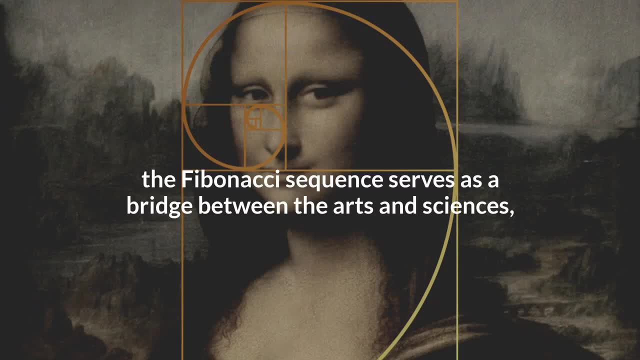 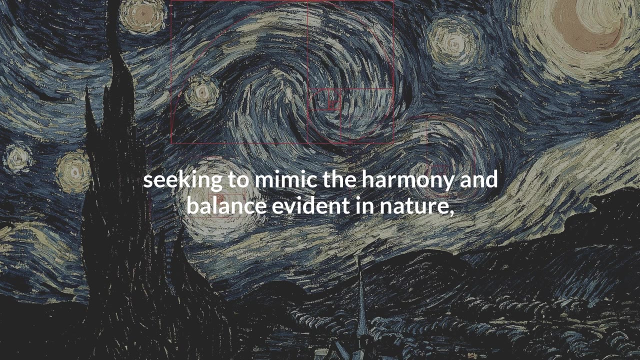 Moreover, the Fibonacci sequence serves as a bridge between the arts and sciences, illustrating how deeply interconnected our world is. Architects and artists have long drawn inspiration from its proportions, seeking to mimic the harmony and balance evident in nature, From the architectural wonders of ancient civilizations to the masterpieces of Renaissance art. 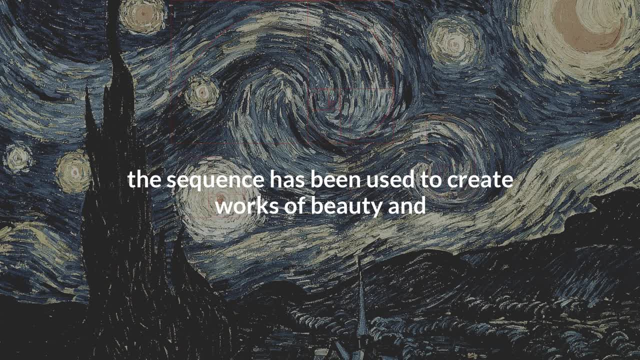 the sequence has been used to create works of beauty and significance that resonate with the natural world. from the architectural wonders of ancient civilizations to the masterpieces of Renaissance art, the sequence has been used to create works of beauty and significance that resonate with the natural world. 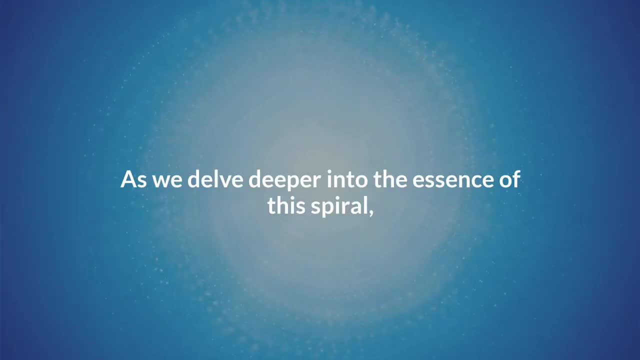 with the natural world. as we delve deeper into the essence of this spiral, we uncover its role as a master key to understanding the cosmos's intricate design and our own existence within it. this spiral is not just a pattern, but a revelation manifesting the golden ratio phi, esteemed throughout history as the epitome of beauty and harmony. 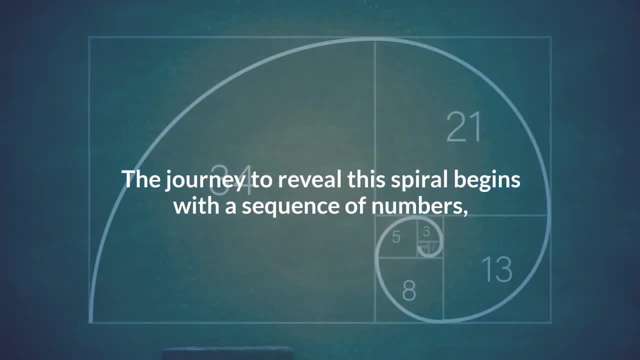 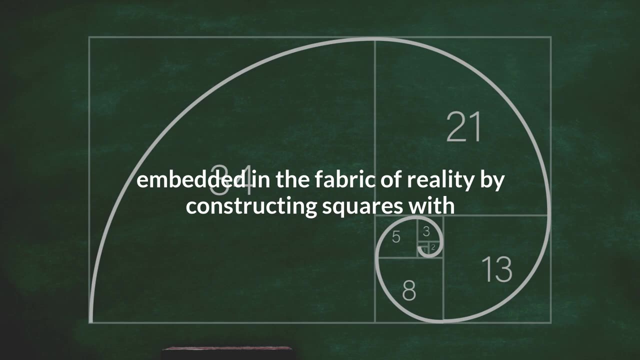 the journey to reveal this spiral begins with a sequence of numbers, each a beacon, leading us to the discovery of an extraordinary pattern embedded in the fabric of reality. by constructing squares with sides corresponding to fibonacci numbers and inscribing quarter circles within these squares, we witness the emergence of a spiral that echoes the natural order of the universe. 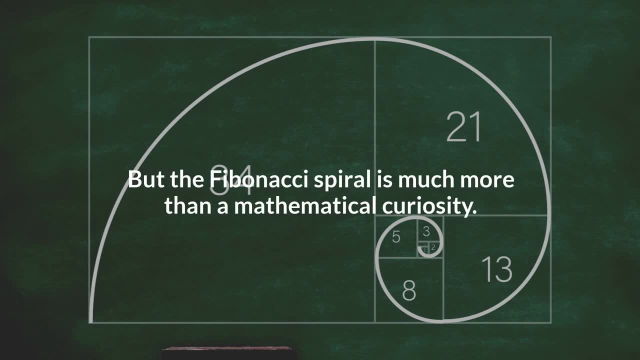 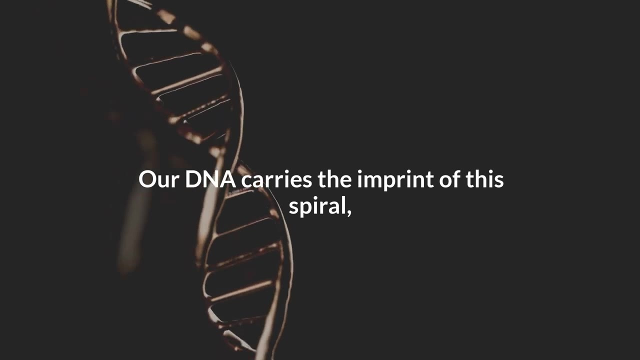 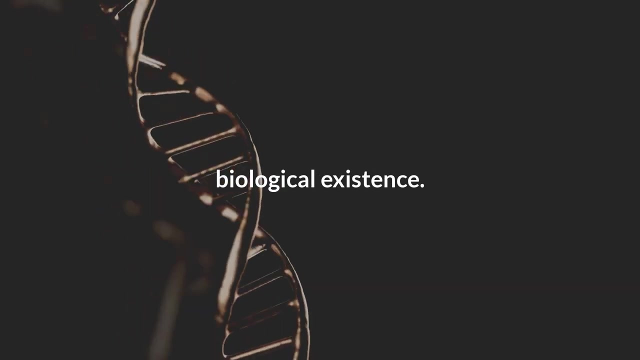 but the fibonacci spiral is much more than a mathematical curiosity. it is a bridge between the abstract and the tangible, a visual expression of growth and evolution, the very essence of life itself. our dna carries the imprint of this spiral, winding into the double helix structure that is the cornerstone of biological existence. this, again, is a corroboration of the spiral's 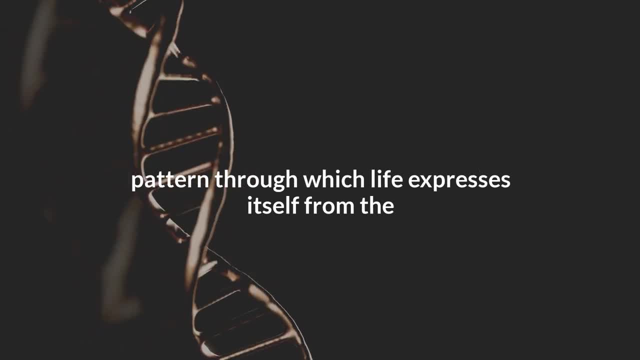 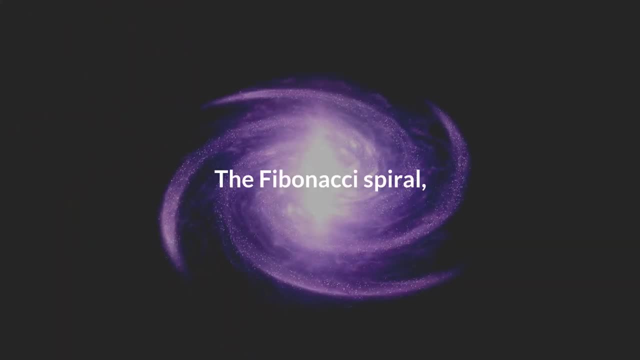 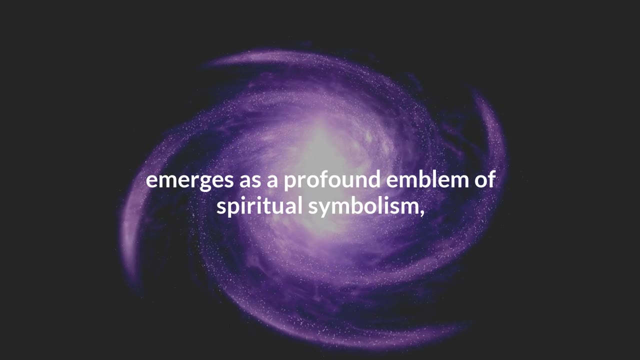 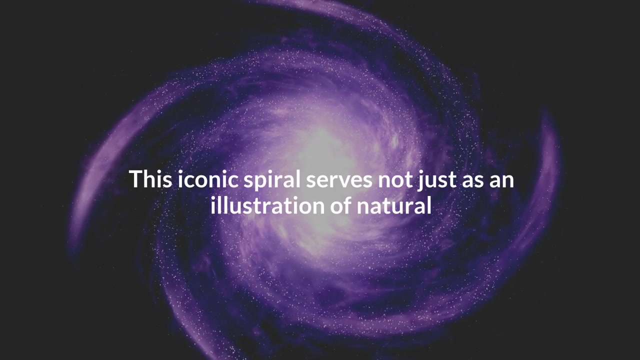 creator leicester. in the literature of georgia, theон fowler is a philosopher and anatomist, a character of the universe. the methods of creation, of programme of evolution, the energy of evolution, the body and the mind are part of this spiral and one of the key elements. 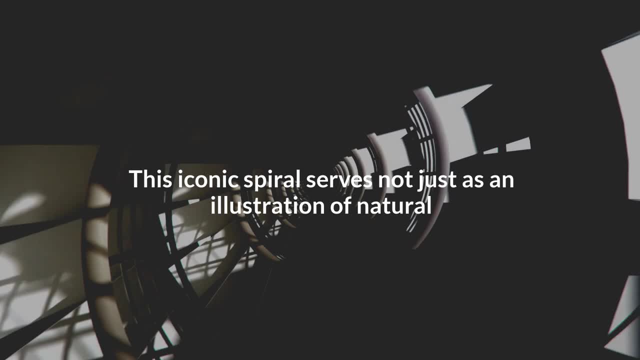 of the model of the gym is the incredible sense of self. that is the spiritual presence. that is a principle, I think. a werewolf's body is a mystery, something which has been depicted over and over and in the past, and when we think through it, we take into account what we see in the memory and to view it. 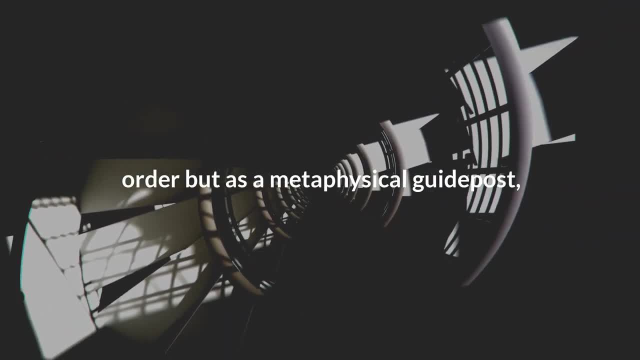 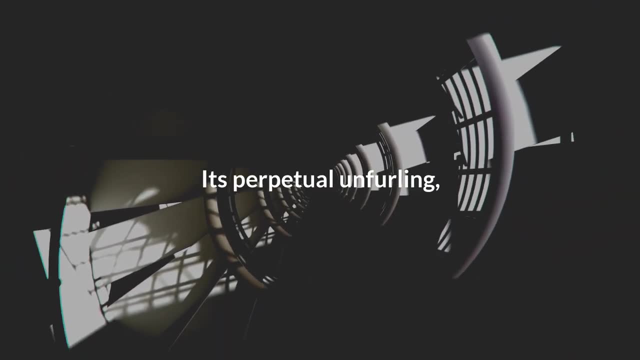 as a naturalDIY, and it is a natural reality that has been acquired by the ancient phoenix, which is the but as a metaphysical guidepost, illuminating the spiritual journey inherent to the human experience, Its perpetual unfurling from the core to the vastness of the universe. 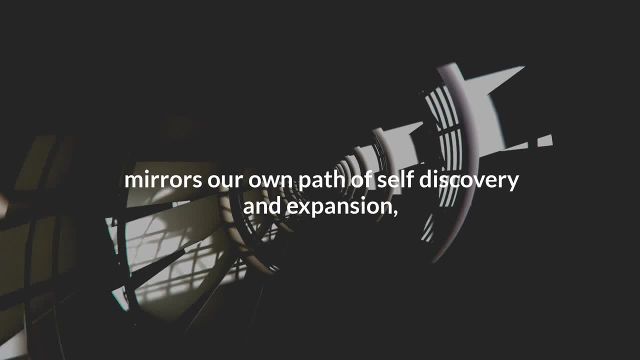 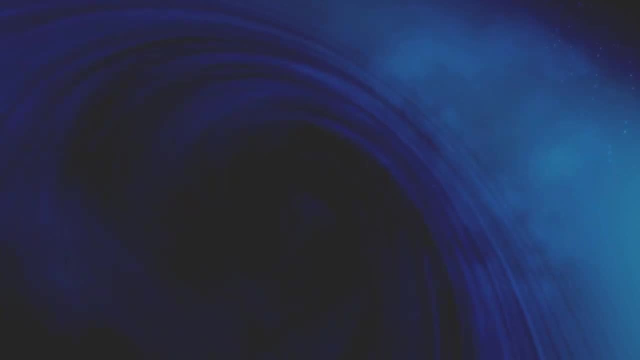 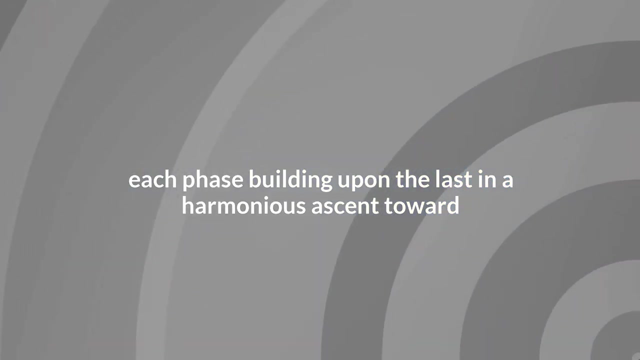 mirrors our own path of self-discovery and expansion, embodying principles of harmony, balance and infinite growth. Within the graceful curves of the Fibonacci spiral, we find a reflection of the spiritual axiom that life is a series of interconnected cycles, each phase building upon the last in a harmonious ascent toward enlightenment. 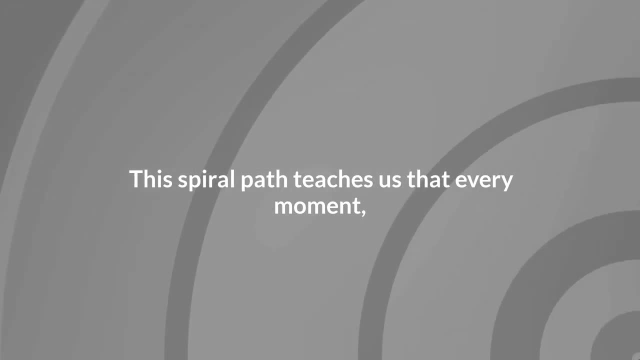 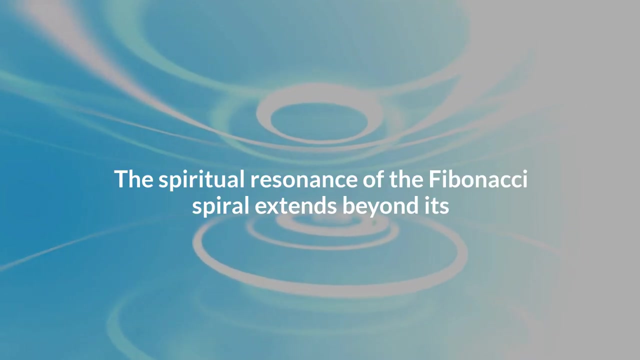 This spiral path teaches us that every moment, every challenge and every triumph is a step on the journey toward understanding our place in the cosmos. It underscores the truth that we are not mere spectators in the universe, but integral components of its vast, intricate design. The spiritual resonance of the Fibonacci spiral. 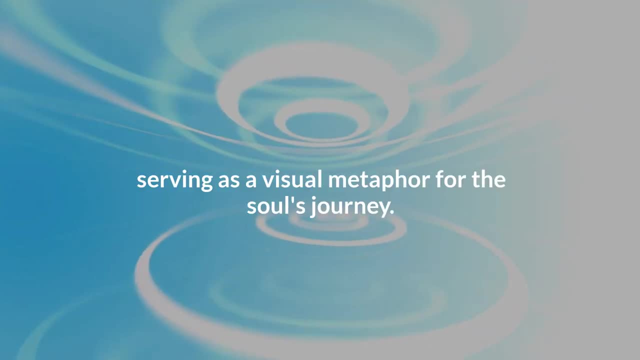 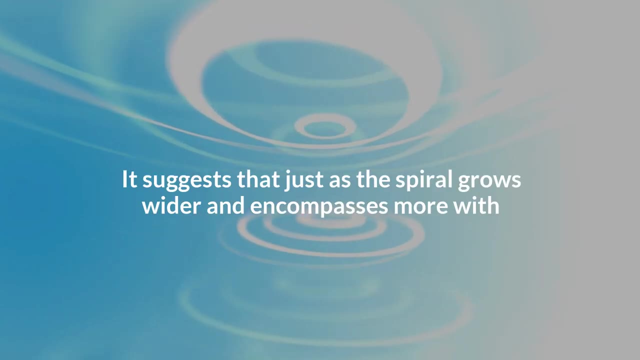 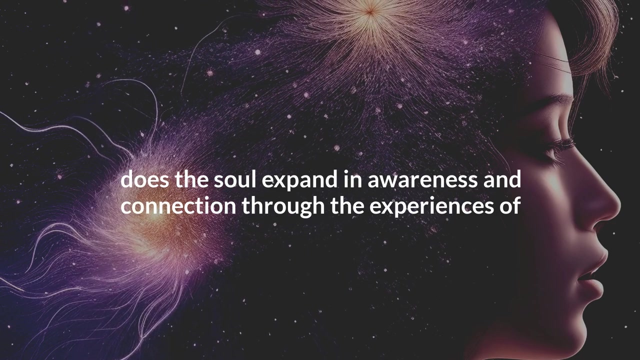 extends beyond its geometric form. serving as a visual metaphor for the soul's journey, It suggests that just as the spiral grows wider and encompasses more with each turn, so too does the soul expand in awareness and connection through the experiences of life. This concept, 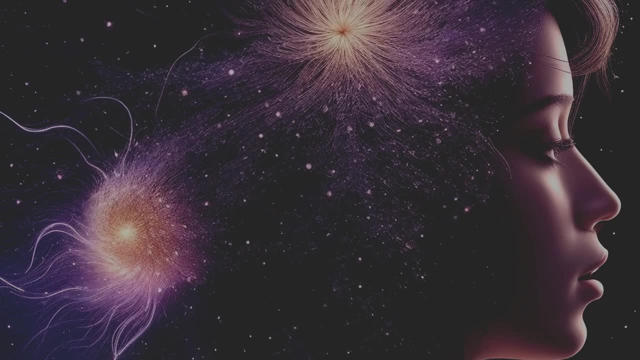 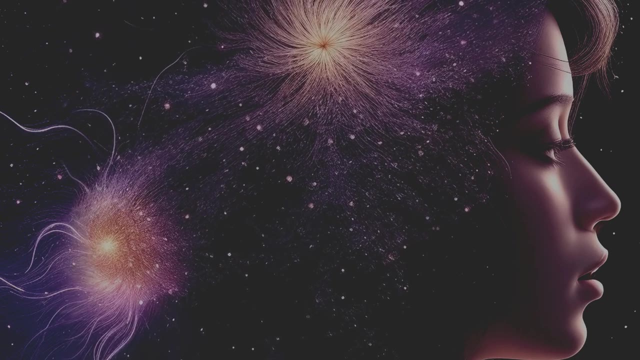 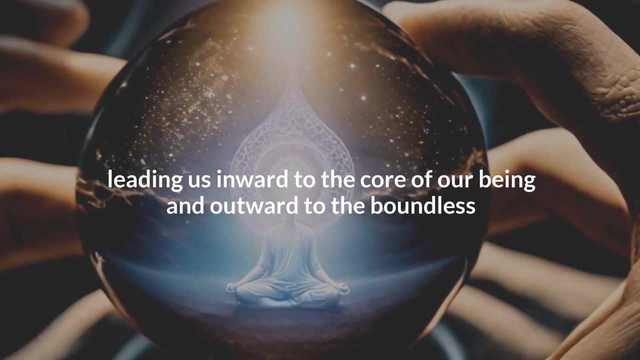 resonates deeply with those on a spiritual path, offering a symbolic representation of personal evolution and the pursuit of higher consciousness. As we meditate on the significance of the Fibonacci spiral, visualizing its path leading us inward, to the core of our being, and outward, to the boundless, 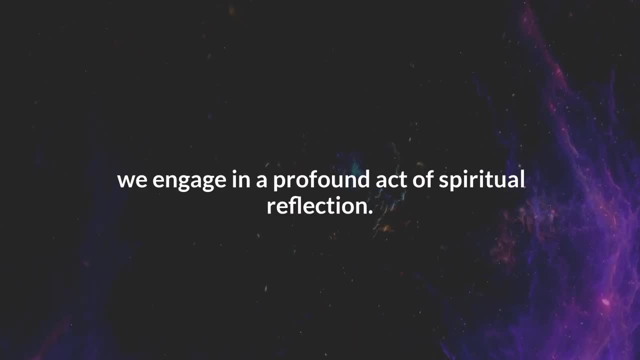 possibilities of the universe, we engage in a profound act of spiritual reflection. This meditation allows us to find our place in the spiritual world and to find our place in the natural order, fostering a sense of peace and belonging. It reminds us that our lives are woven. 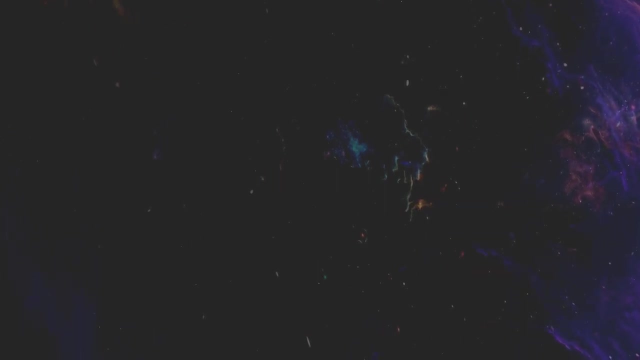 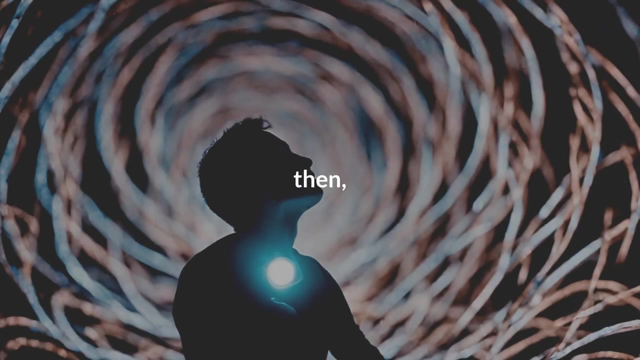 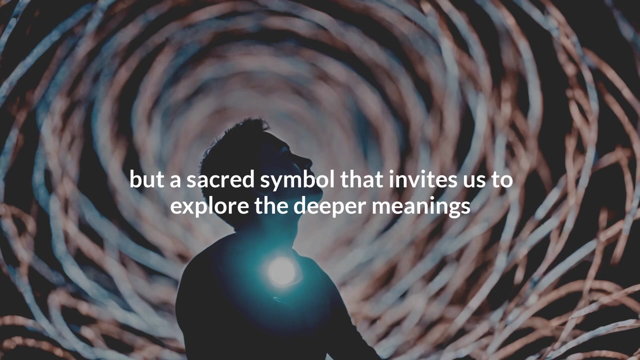 from the same fabric as the stars and galaxies, and that our growth and progression are part of a greater divine pattern. This spiral, then, is not merely a pattern to be observed in the physical realm, but a sacred symbol that invites us to explore the deeper meanings of existence. 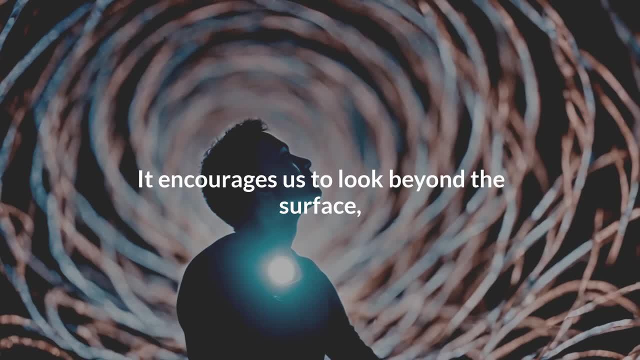 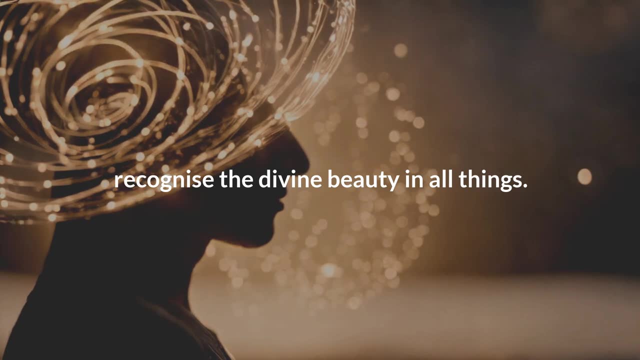 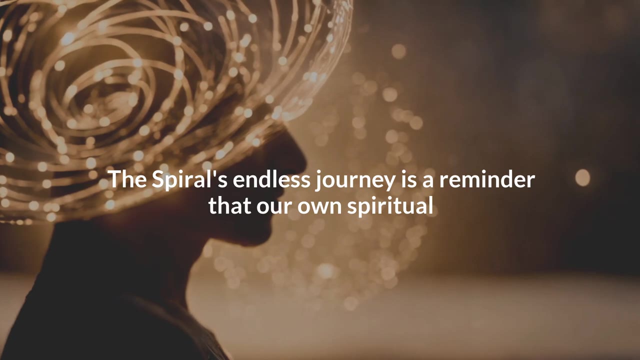 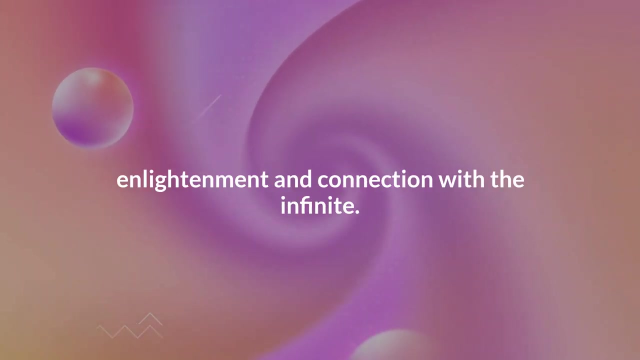 It encourages us to look beyond the surface, to see the unity that underpins diversity, and to recognize the divine beauty in all things. The spiral's endless journey is a reminder that our own spiritual quest is never complete, but is an ongoing voyage of discovery, enlightenment and connection with the infinite. 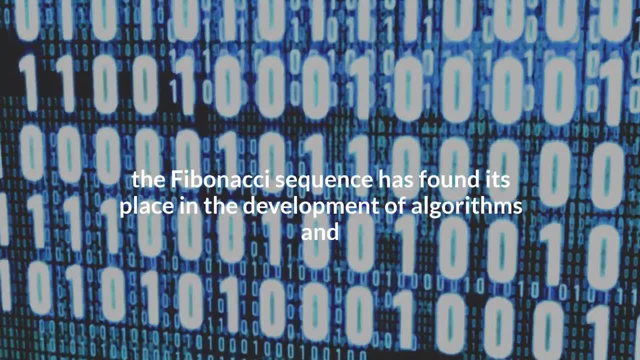 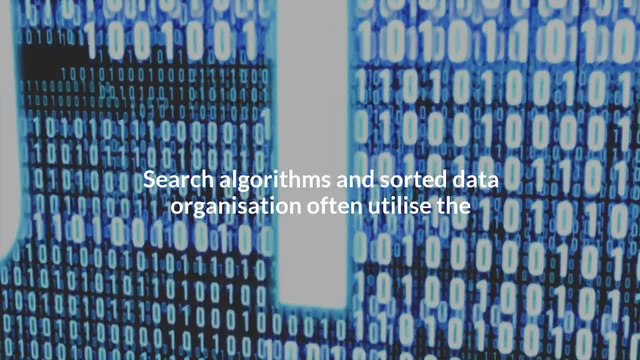 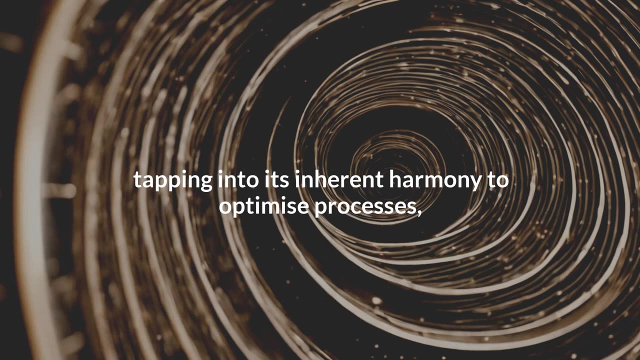 In the field of spiritual reflection. the spiral is a reminder that we are an infinite source of computer science. the Fibonacci sequence has found its place in the development of algorithms and data structures. Search algorithms and sorted data organization often utilize the sequence's efficiency, tapping into its inherent harmony, to optimize processes. 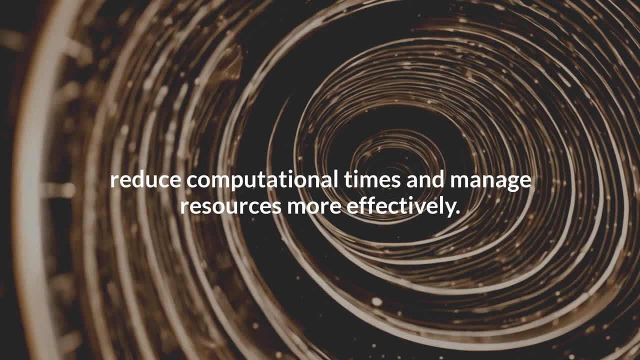 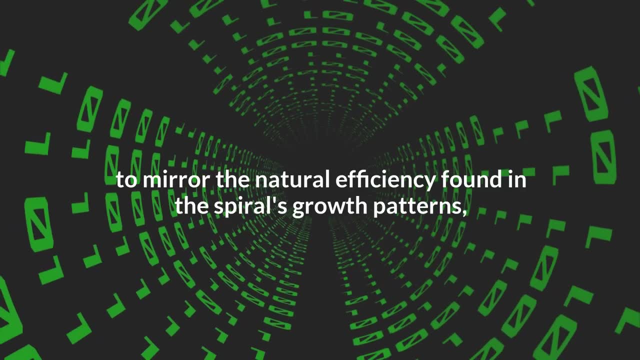 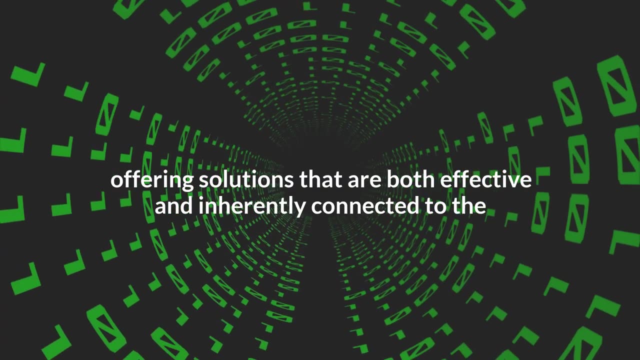 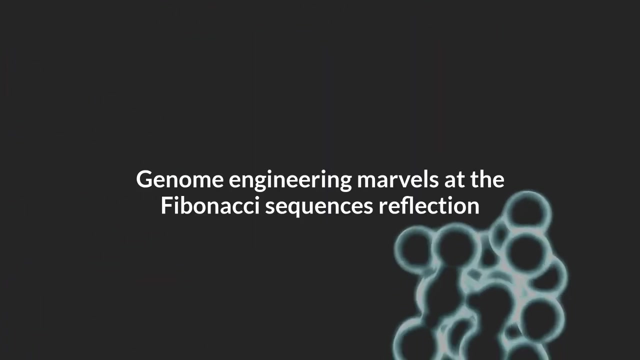 reduce computational times and manage resources more effectively. The elegance of Fibonacci-based algorithms lies in their ability to mirror the natural efficiency found in the spiral's growth patterns, offering solutions that are both effective and inherently connected to the natural logic of the universe. Genome engineering marvels at the Fibonacci sequence's reflection in the very 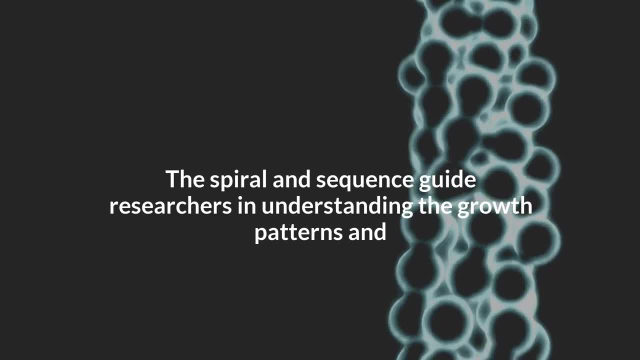 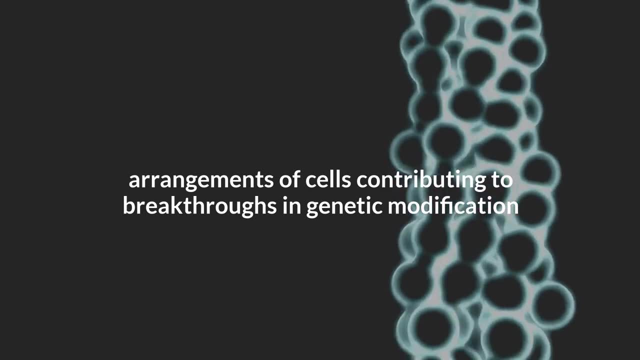 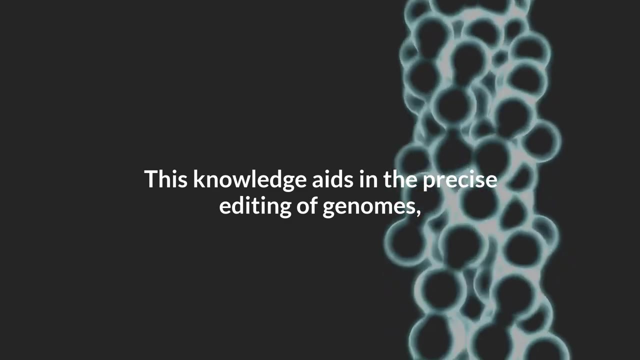 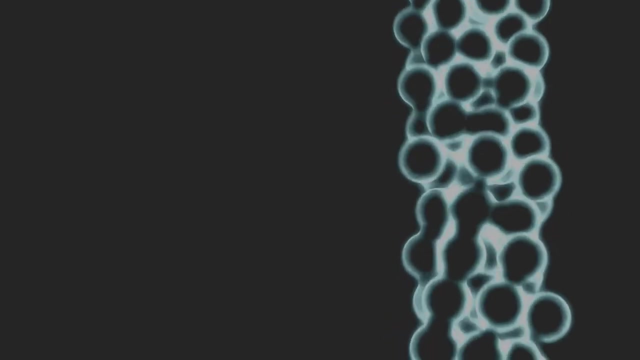 blueprint of life. The spiral and sequence guide researchers in understanding the growth patterns and arrangements of cells, contributing to breakthroughs in genetic modification and therapy. This knowledge aids in the precise editing of genomes, harnessing the sequence's natural efficiency for innovations in medicine and biotechnology. The Fibonacci sequence's role in the distribution. 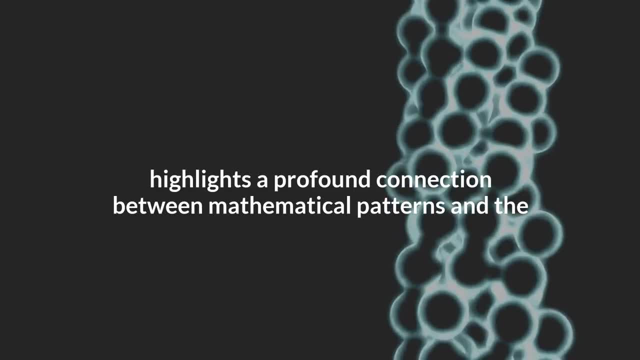 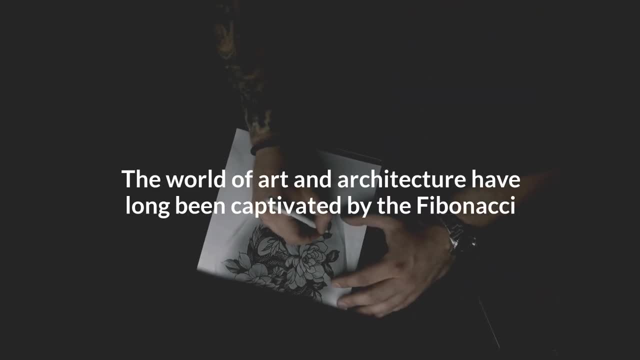 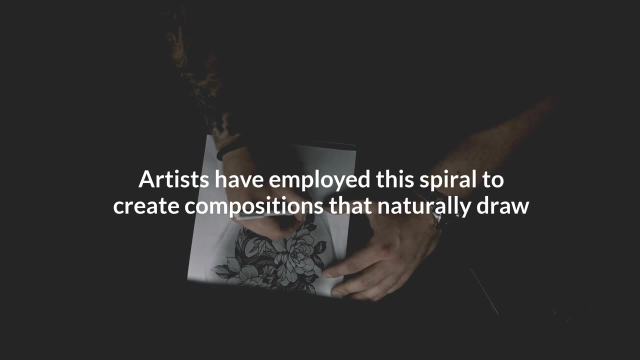 of genes and the structure of proteins highlights a profound connection between mathematical patterns and the fundamentals of life. The world of art and architecture have long been captivated by the Fibonacci Spiral's aesthetic perfection. Artists have employed this spiral to create compositions that naturally draw the viewer's 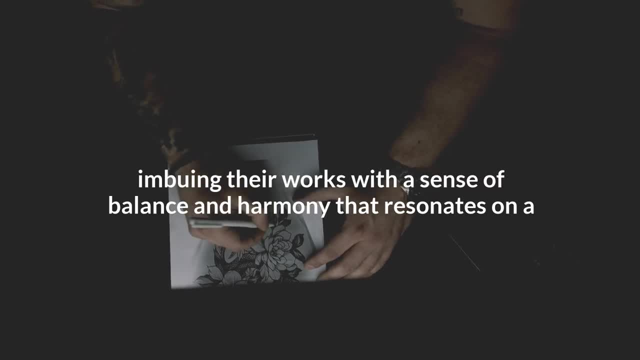 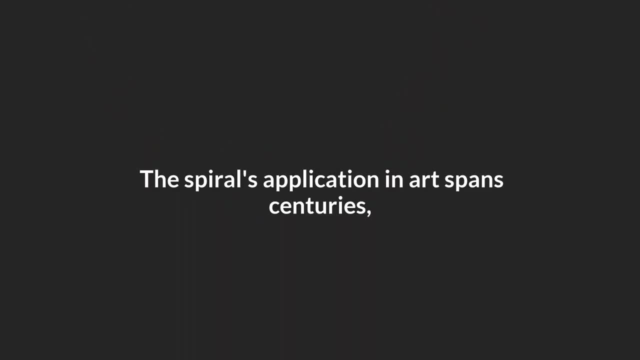 eye, imbuing their works with a sense of balance and harmony that resonates on a deeply intuitive level. The spiral's application in art spans centuries, influencing the layout of paintings, sculptures and even digital visual effects to evoke beauty and coherence In architecture. 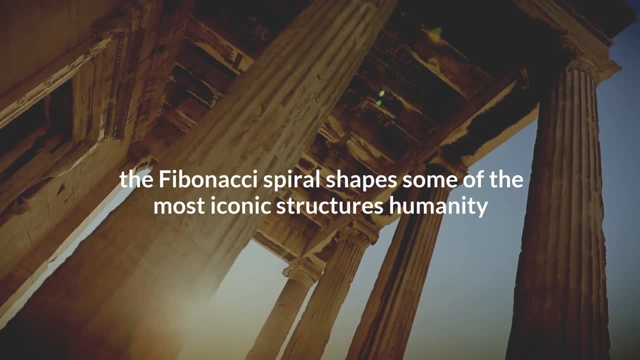 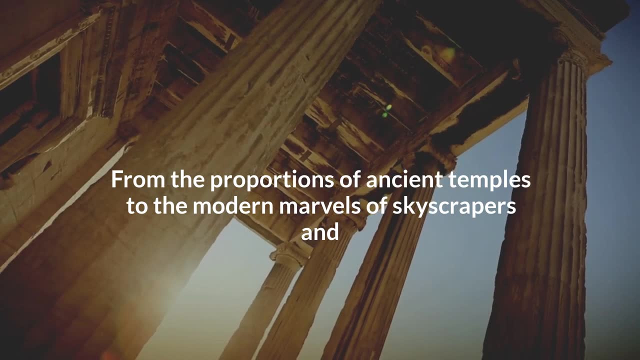 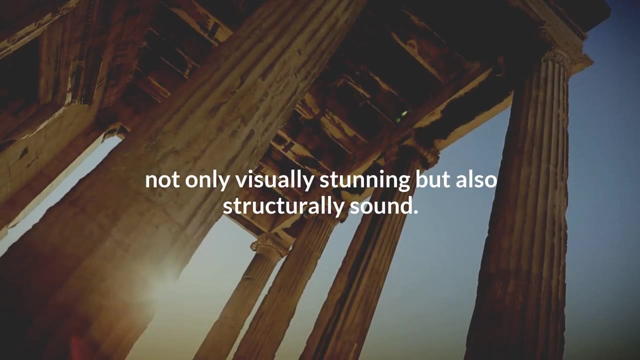 the Fibonacci Spiral shapes some of the most iconic structures humanity has ever constructed, From the proportions of ancient temples to the modern marvels of skyscrapers and bridges. architects have used the spiral and sequence to achieve an aesthetic that is not only visually stunning but also structurally sound. 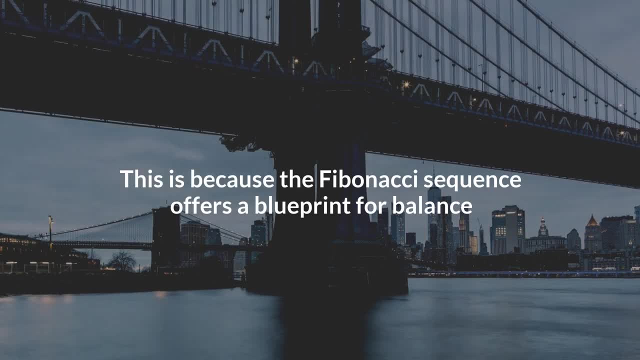 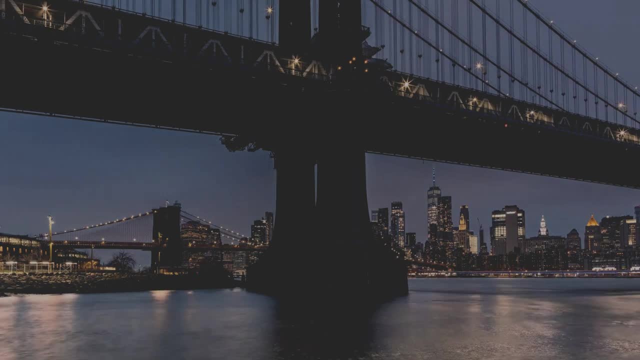 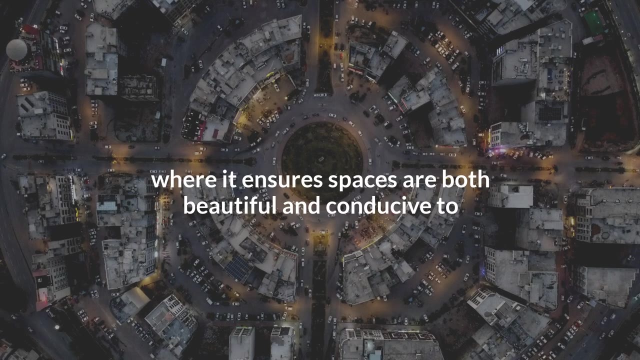 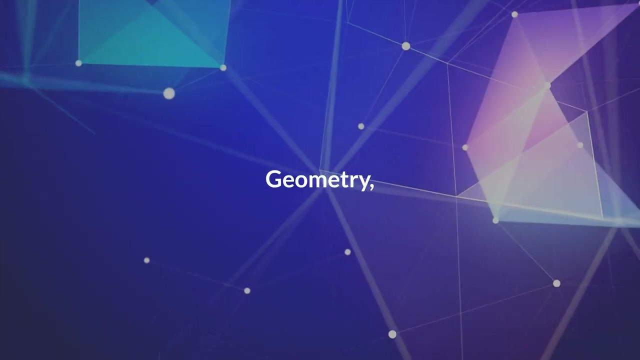 This is because the Fibonacci sequence offers a blueprint for balance and strength, reflecting the harmony between form and function. The spiral's influence is evident in the design of buildings and urban layouts, where it ensures spaces are both beautiful and conducive to human activity. Geometry, the foundational language of both art and science, embraces 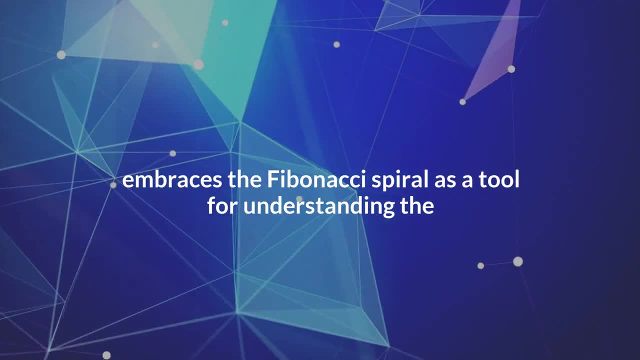 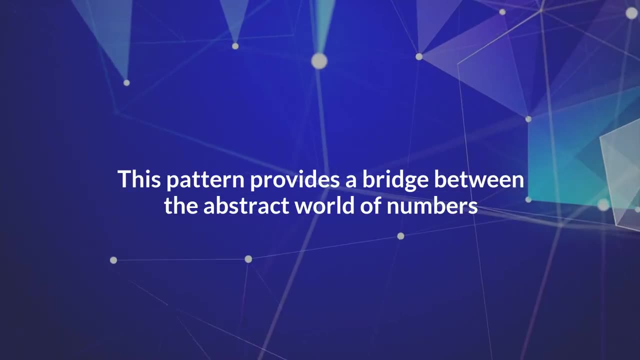 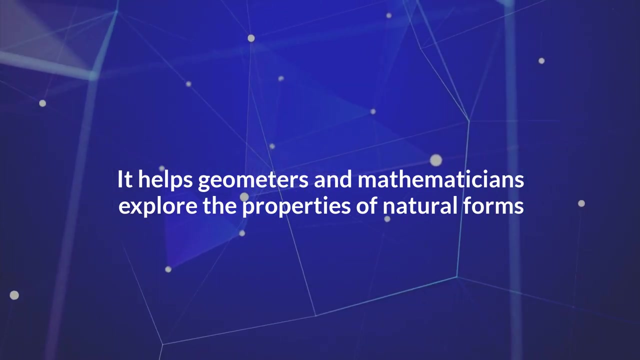 the Fibonacci Spiral in a way that is both beautiful and conducive to human activity. The Fibonacci Spiral is a tool for understanding the principles of shape and space. This pattern provides a bridge between the abstract world of numbers and the tangible reality we navigate daily. It helps geometers and mathematicians explore the properties of 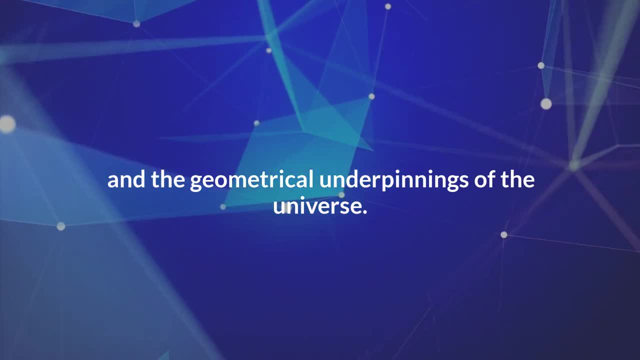 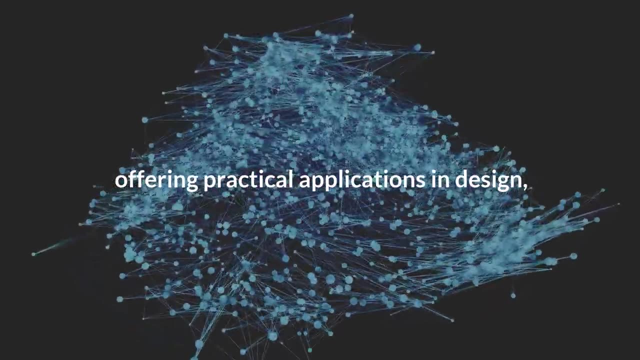 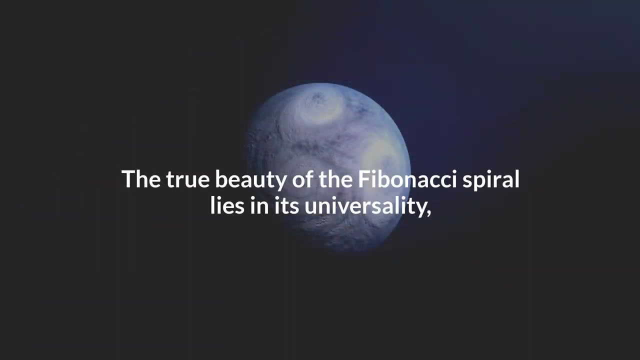 natural forms and the geometrical underpinnings of the universe. The spiral has propelled advancements in theoretical mathematics while also offering practical applications of the hinting and bashing of the style of Earth. This series of later inspirations providesコh represions for design, engineering and technology. 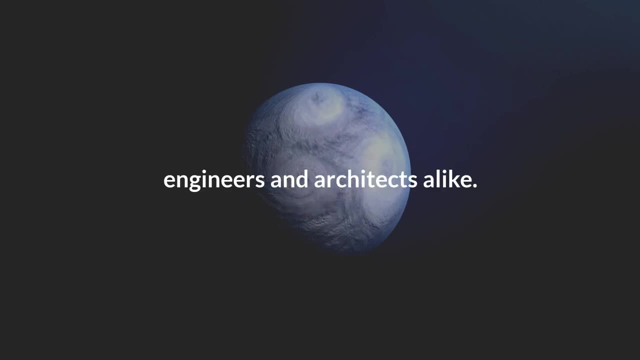 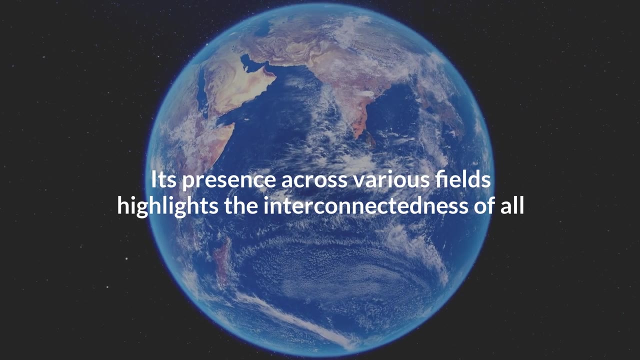 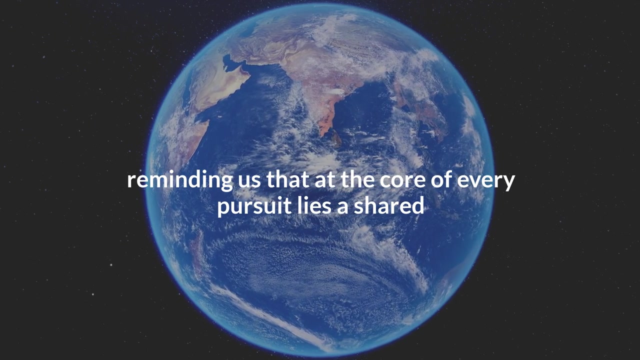 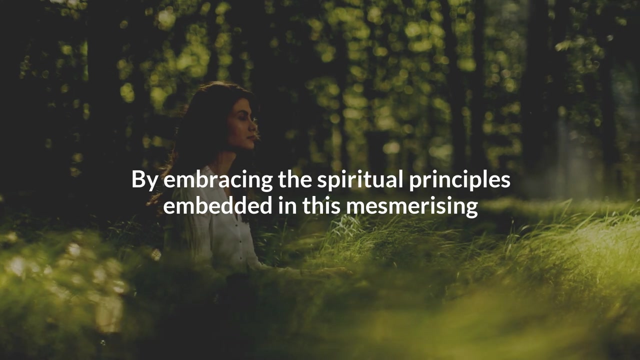 The true beauty of the Fibonacci Spiral lies in its universality – a principle that transcends the boundaries between disciplines, offering insights and inspiration to scientists, artists, reminding us that at the core of every pursuit lies a shared quest for understanding and harmony. by embracing the spiritual principles embedded in this mesmerizing spiral, you can unlock the power. 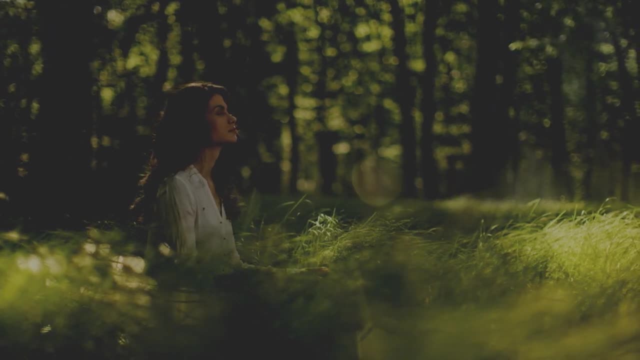 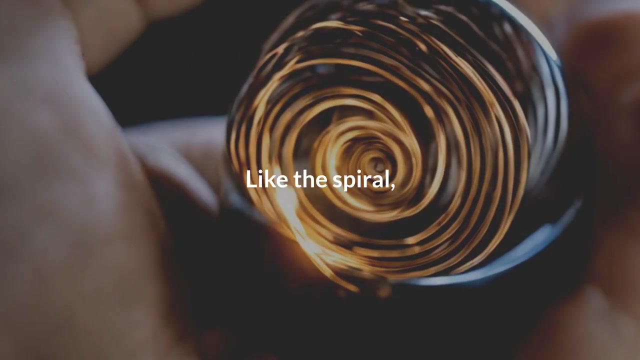 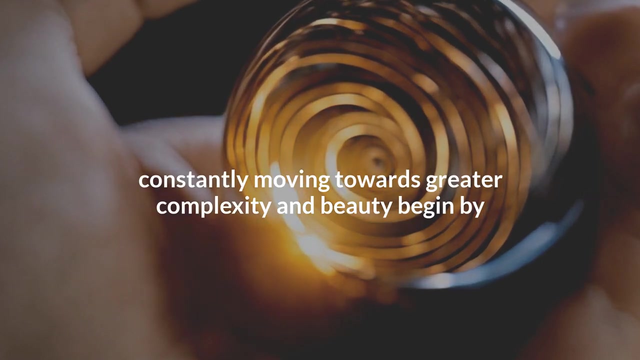 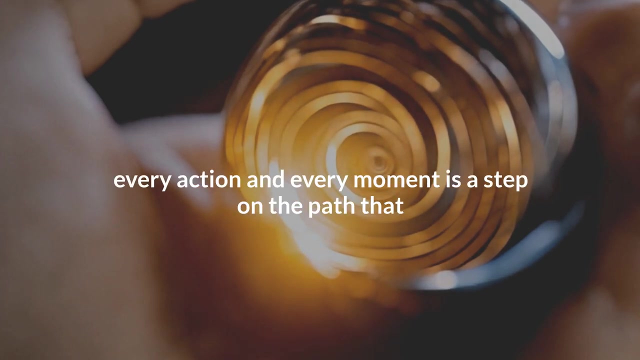 to manifest the life you've always dreamed of. at the heart of the fibonacci spiral lies the essence of expansion and progression. like the spiral, your journey is ever evolving, constantly moving towards greater complexity and beauty. begin by visualizing your life as part of this divine geometry, where every thought, every action and every moment is a step on the path that 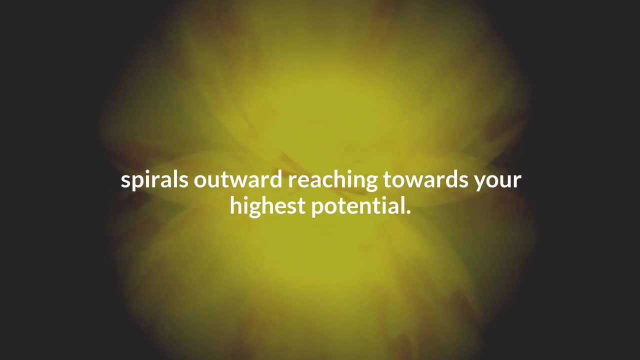 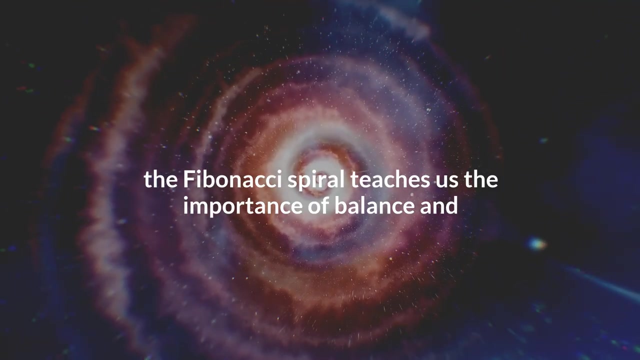 spirals outward, reaching towards your highest potential. recognize that you are not separate from the universe, but a a vital part of its infinite fabric. woven from the same patterns that spiral in the stars and dance in the dna strands, the fibonacci spiral teaches us the importance of balance and proportion, principles that are crucial. 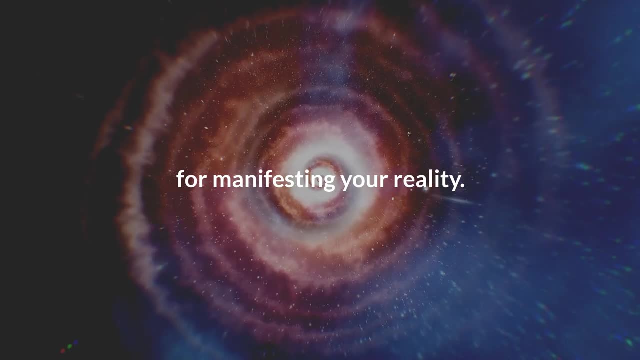 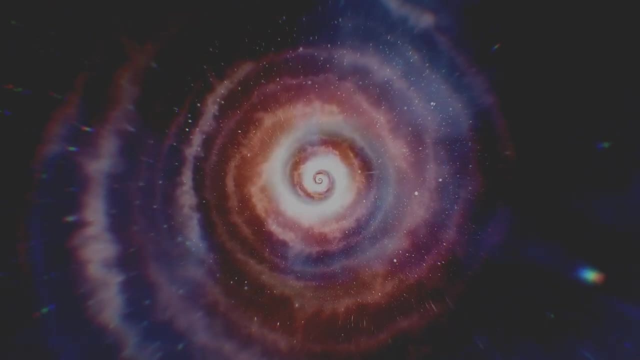 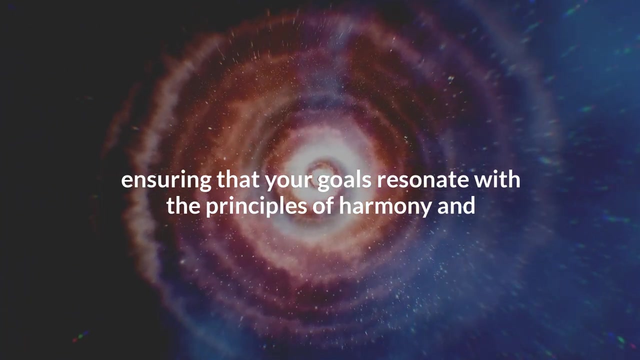 when setting intentions for manifesting your reality. as you contemplate your desires, align them with the now, the natural flow of the universe. consider not just the outcome but the journey there, ensuring that your goals resonate with the principles of harmony and growth by setting intentions that mirror the balance found in the spiral. 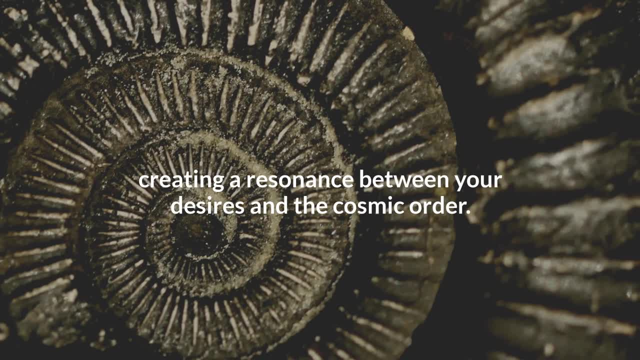 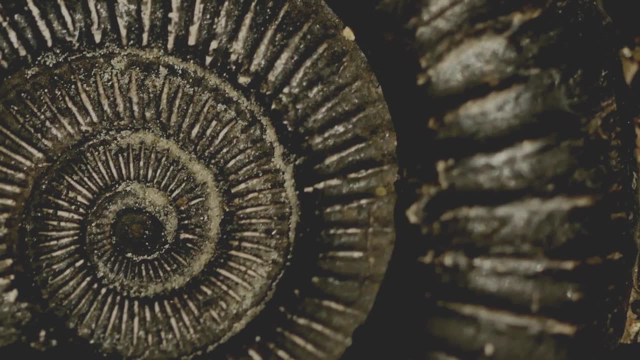 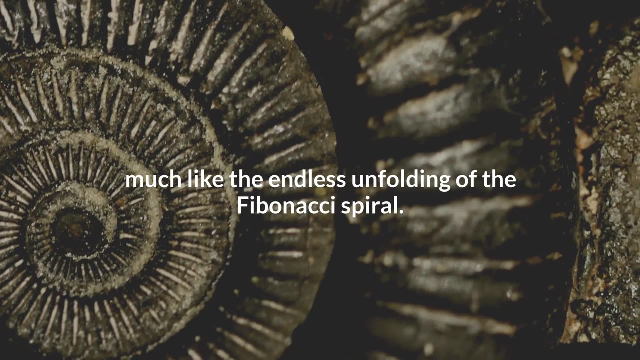 you invite the universe to support your aspirations, creating a resonance between your desires and the cosmic order. manifestation is not a single act, but a process of continuous growth and realising that you are really in this process of revitalisation in the beautiful world we all Oui. 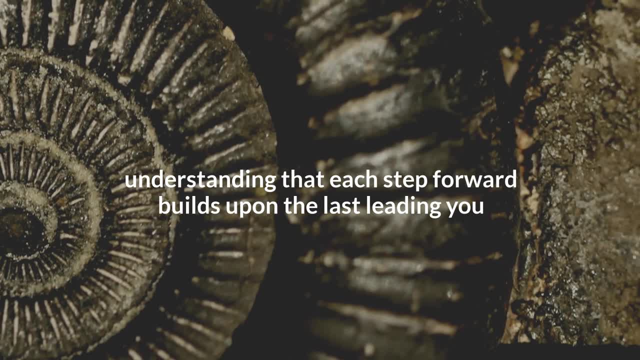 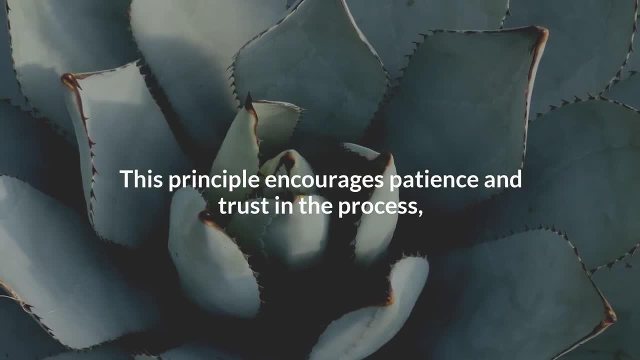 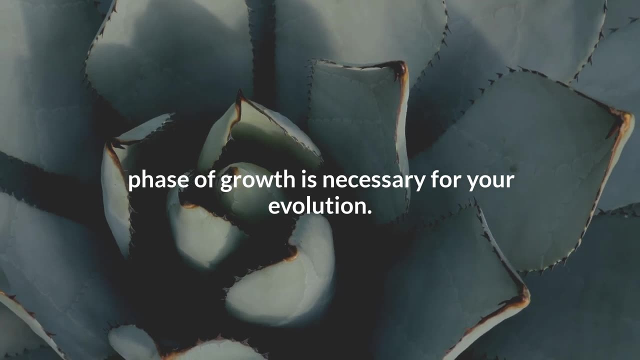 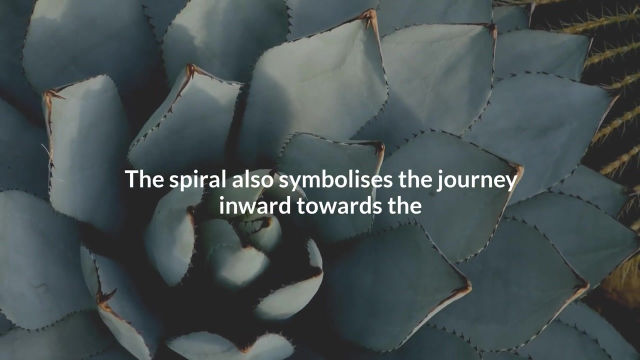 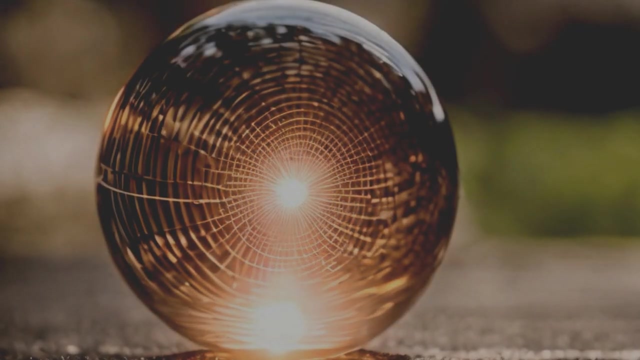 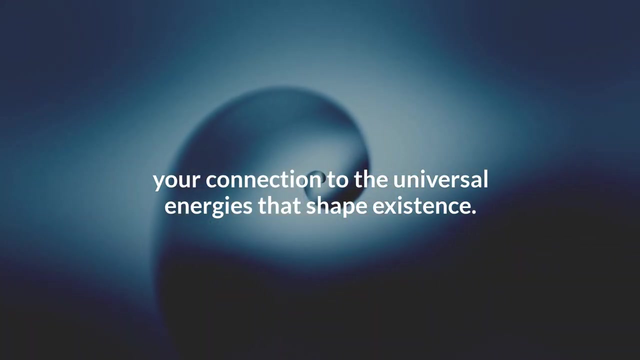 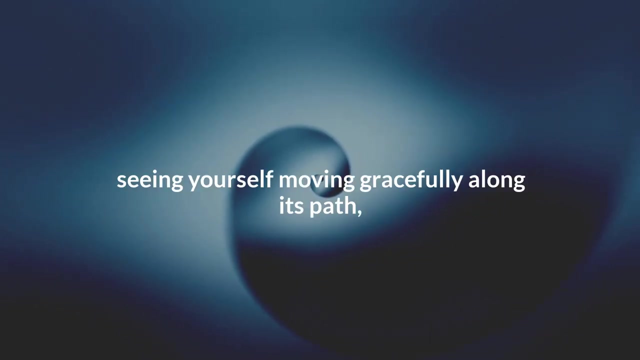 with a music wrote by it can. The spiral also symbolizes the journey inward towards the essence of your being, where true manifestation begins. Regular reflection and meditation on the Fibonacci spiral can deepen your connection to the universal energies that shape existence. Visualize the spiral in your mind's eye, seeing yourself moving gracefully along its path. 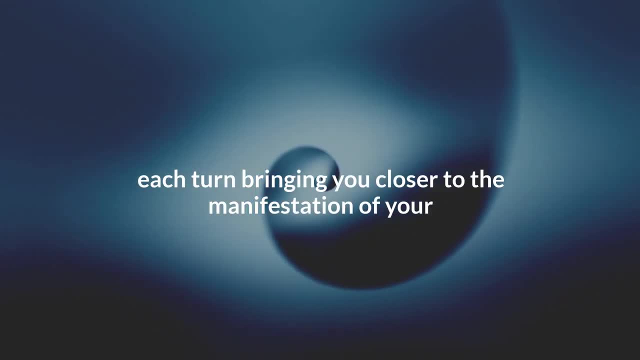 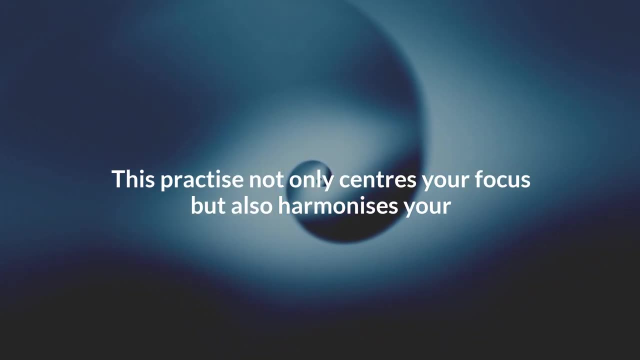 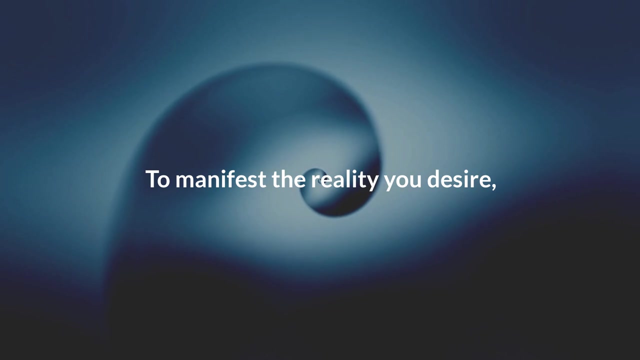 each turn, bringing you closer to the manifestation of your desires. This practice not only centers your focus, but also harmonizes your energy with the creative forces of the universe To manifest the reality you desire. embody the qualities of the Fibonacci spiral in your daily life. 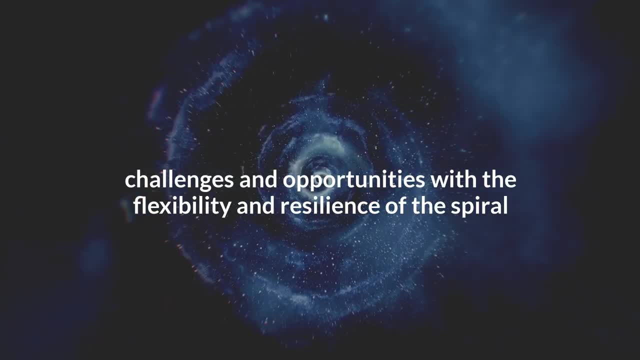 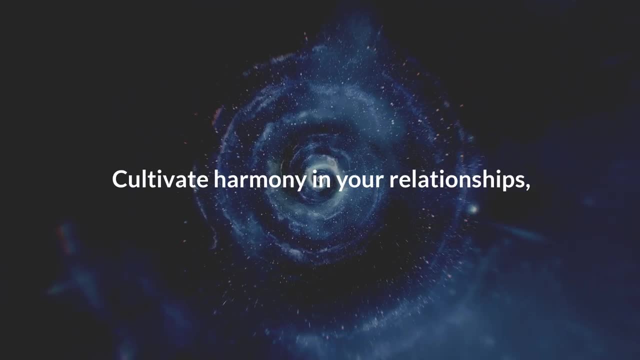 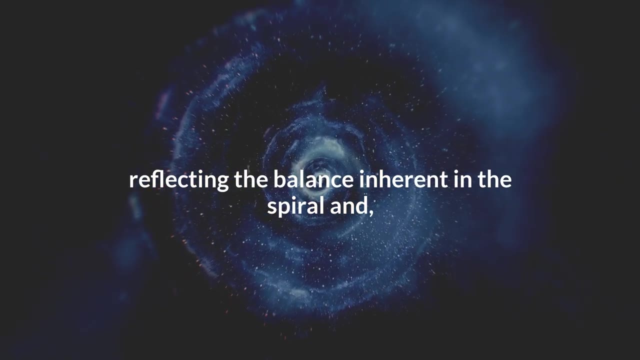 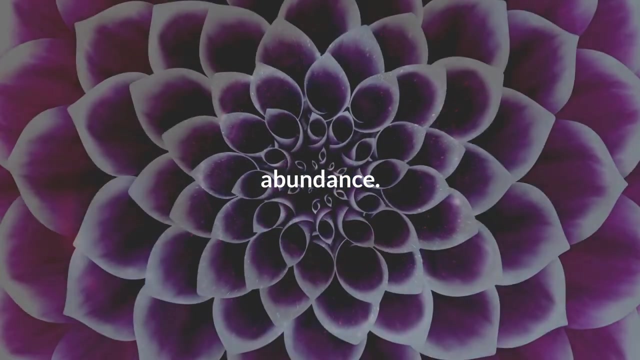 Approach challenges and opportunities, with the flexibility and resilience of the spiral, adapting and growing with it. Cultivate harmony in your relationships, your environment and your inner world, reflecting the balance inherent in the spiral. And, most importantly, allow the spiral's infinite nature to inspire a mindset of abundance. 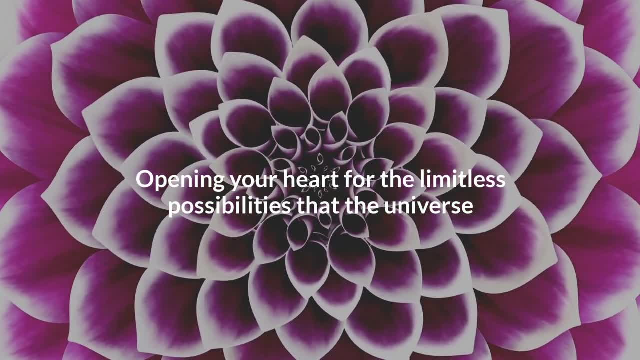 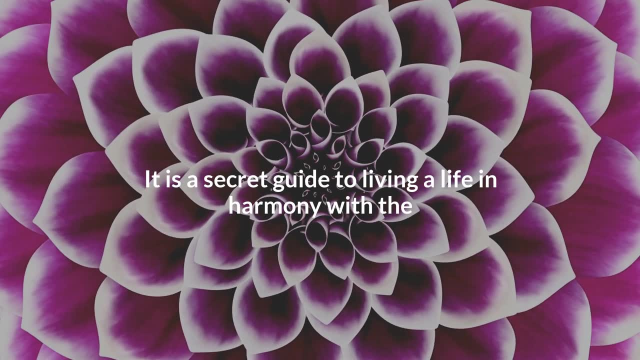 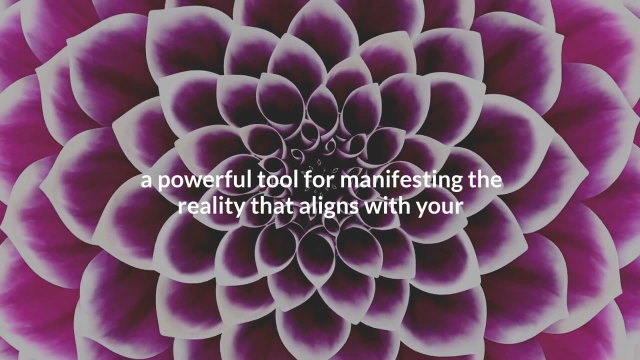 opening your heart to the limitless possibilities that the universe offers. The Fibonacci spiral is more than a symbol. It is a secret guide. It is a tool to living a life in harmony with the cosmos, a powerful tool for manifesting the reality that aligns with your deepest desires.